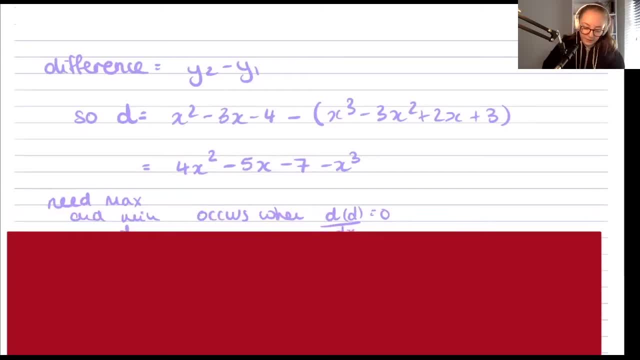 like I said earlier, this occurs when the first derivative of our equation is equal to zero. A slight oversight from me. I called our equation d- and we often use the notation d- something, ydx, where something is our function, And I call that function d, So it's dd by dx, which is slightly. 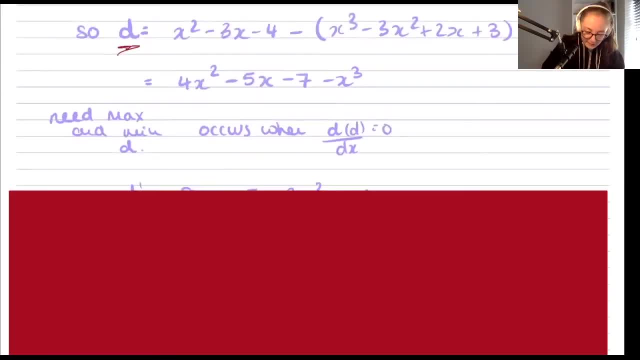 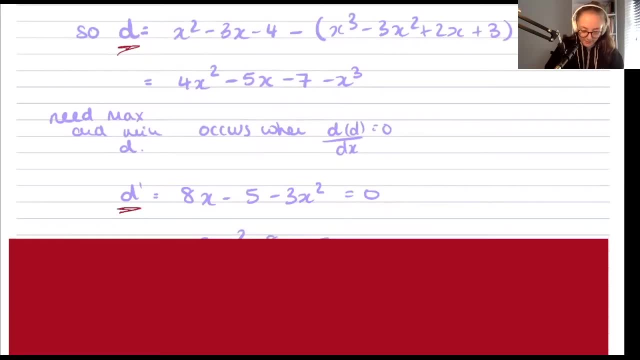 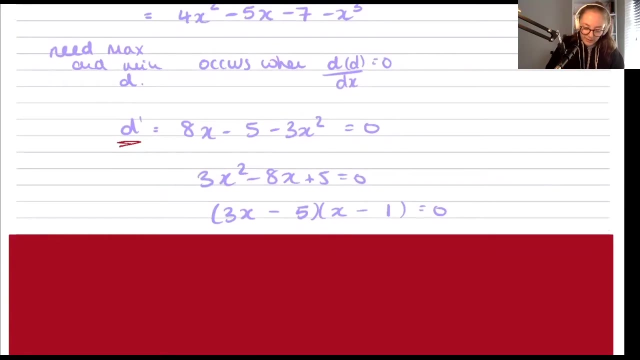 confusing, but just ignore that. So if we take dd by dx or d prime, as I told you about the notation earlier, and then set it to zero, we can rearrange our equation and factorize it to get two values of x, And these values are one and five over three. That's all well and good, but we need to know. 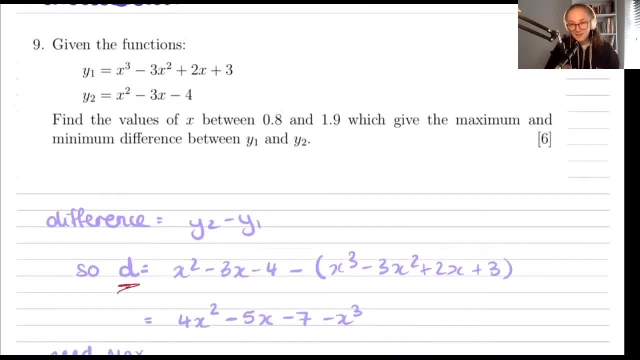 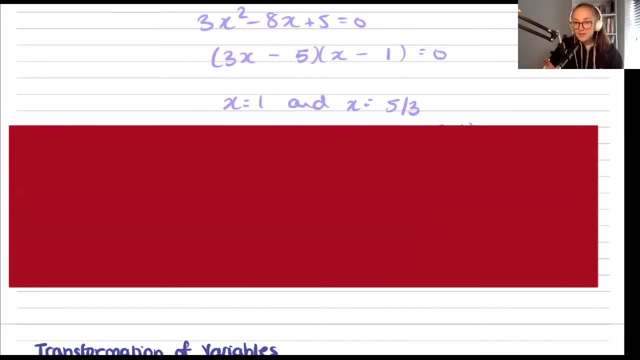 which one is the maximum and which one is the minimum. Otherwise we are unlikely to achieve all six of the marks. So the next step. you can choose to do different things for this, but you can either take the second derivative and see the result. 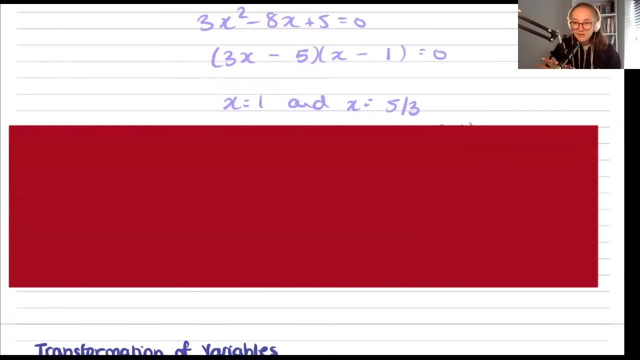 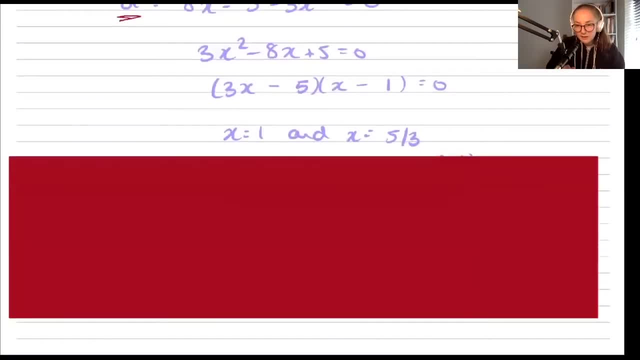 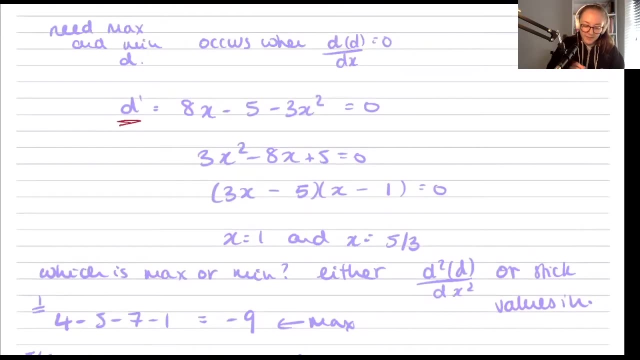 See the signs of the second derivative. But this can be slightly messy depending on which way around you put your y2 and your y1, because that will change the sign in itself. So I decided to do it a slightly simpler way by just sticking in these values into our d. 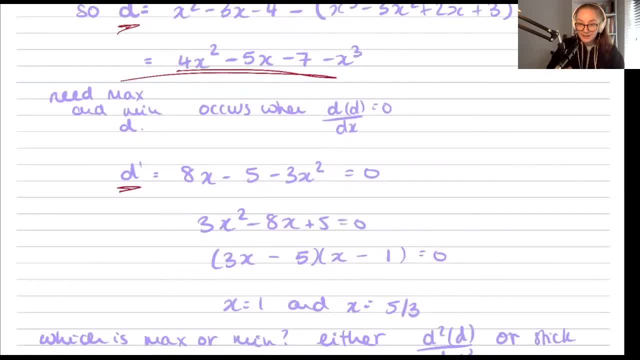 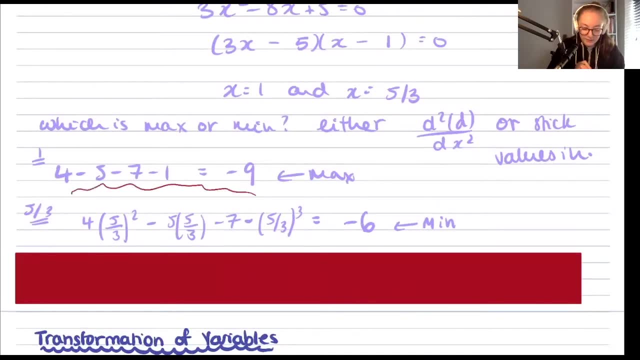 not our d prime. Be careful to stick it into d And then see which one gives you the largest difference and which one gives you the smallest difference. And for one we get a difference of nine And for five over three we get a difference of six minus six, And just in magnitude. 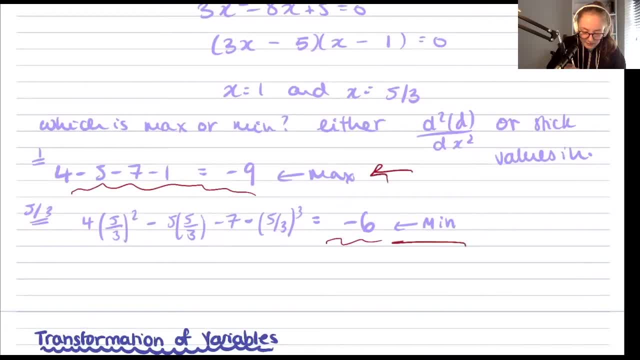 it's clear that this difference is larger than this difference. So that's, when x is one, we have our maximum, And when x is five over three, we have our minimum. So this next topic is transformation of variables, And you kind of just use these skills a lot. 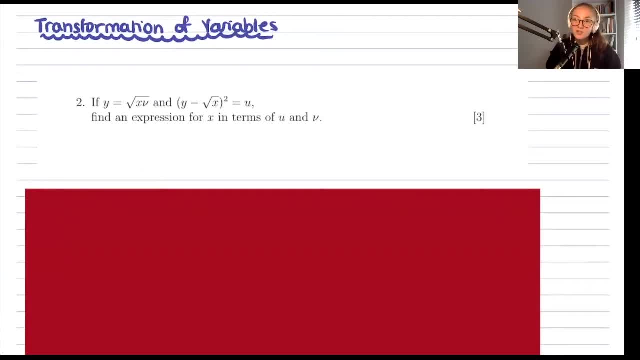 and it's very rare for a question on transformation of variables to just come up. It's more just a skill that you use in other questions. But this is probably the closest question I could find to being transformation of variables And it asks us to come up with an expression for x in terms of u and v only, so we can't involve y. 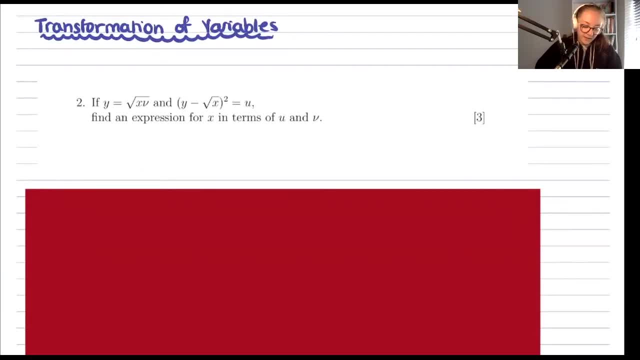 in this expression And we are also given y is root xv and y is root x, y minus root x, all squared. So I would say the easiest thing to do here, because it's really easy to just get yourself stuck in knots. 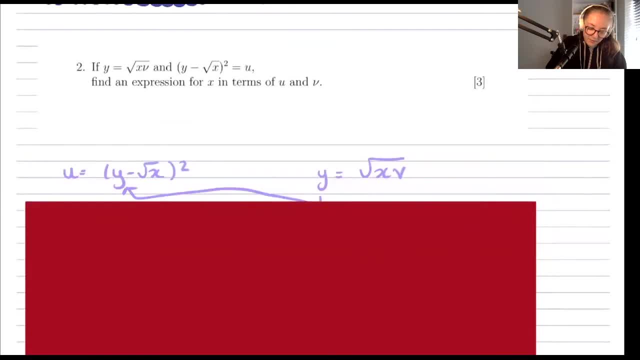 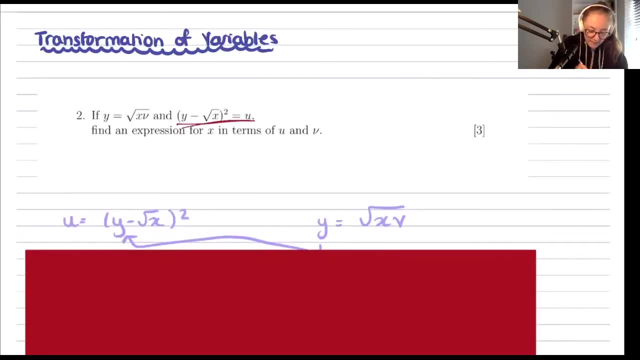 is to just stick in the thing we want to get rid of. So we have an expression involving x here and y, But we just don't want y in this expression. So we could rearrange all this and then get stuck in knots if we wanted to, Or we could just get rid of this y immediately by 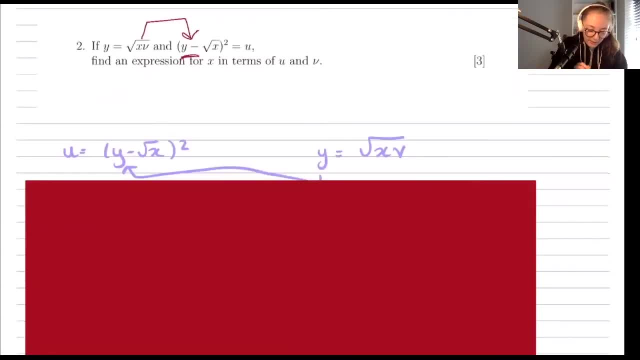 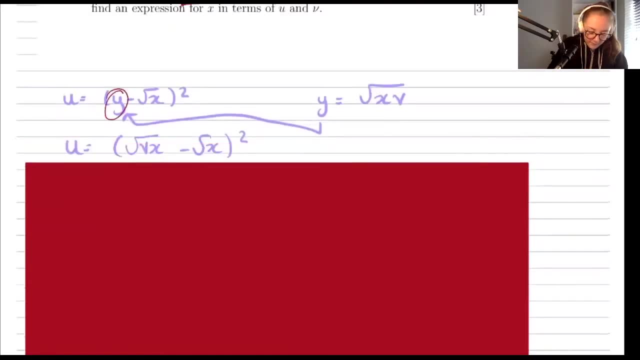 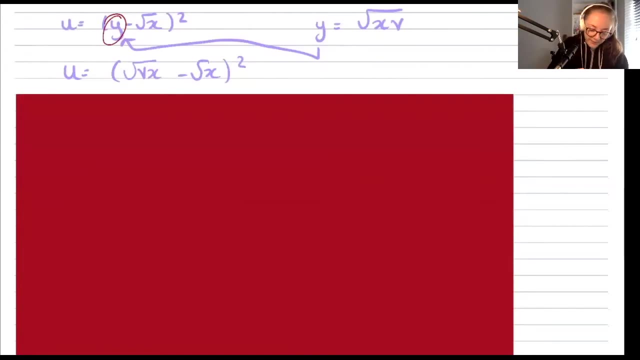 sticking this in. So that's what I've done. I've stuck in y equals root xv into this y here to get u equals root vx minus root x, all squared, And then at this point you can choose to do several different things. You can expand. 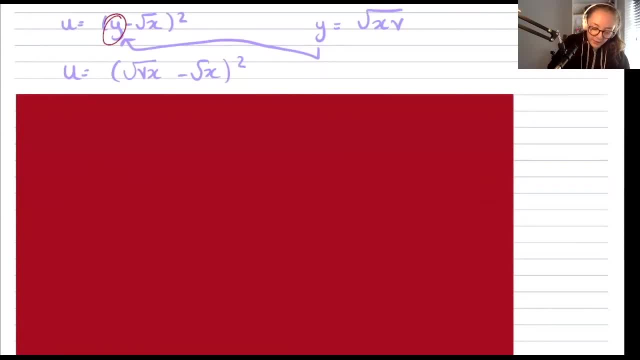 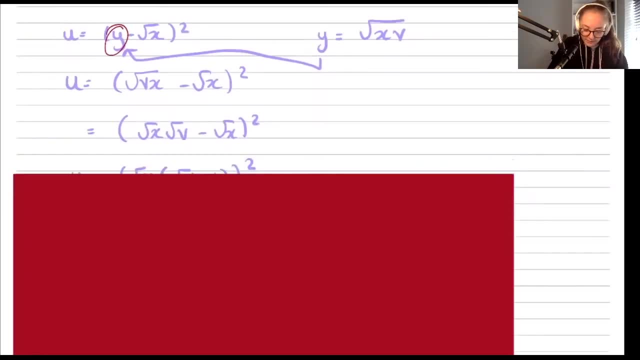 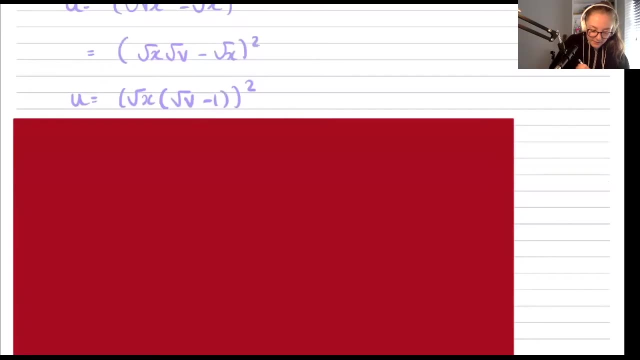 the brackets if you want, but for me I found the easiest thing to do was just to factorise the root x first. So root vx is the same as root x times root v, or root v times root x, whichever way you like. Then I took this root x out, So I factorized that. 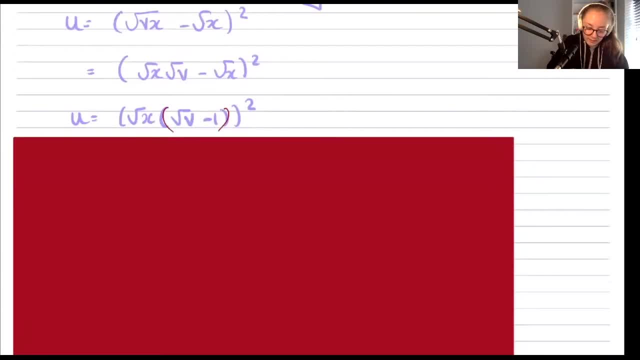 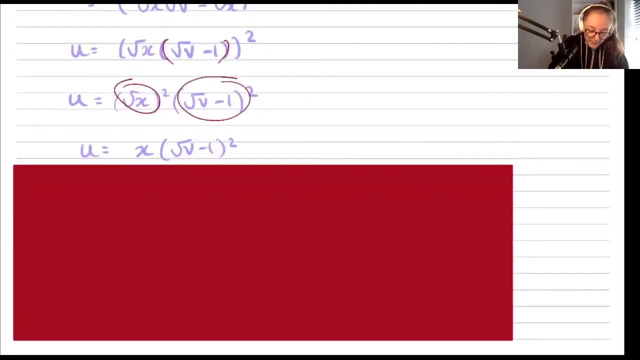 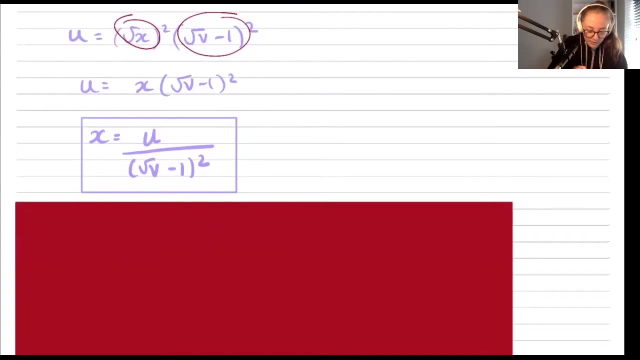 And then when you square two things that are multiplied together, you can just take the square over here and keep the square over here. So then I could square this x and rearrange to get x. is u over root, v minus 1, all squared. 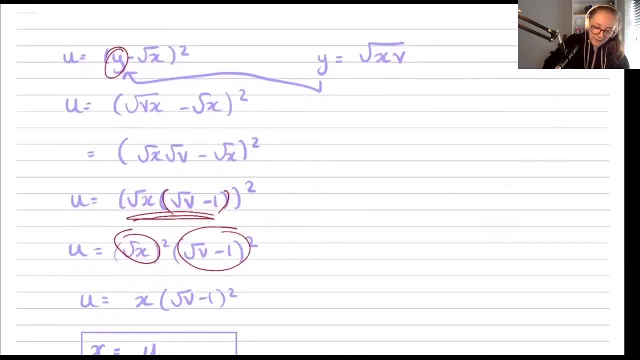 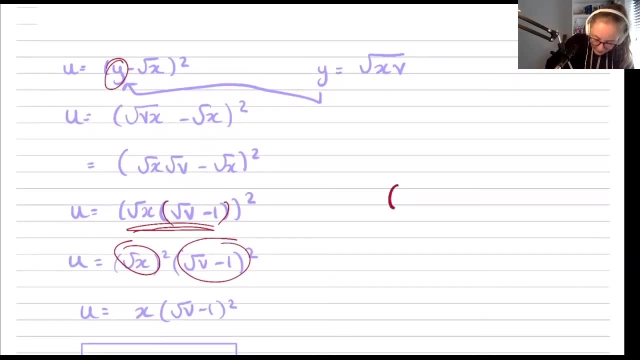 And if you're confused about this step here, then I think probably the best way I can describe this is: okay. so if we have 6 times 3 plus 6 times 2 all squared, then we can factorize that 6. 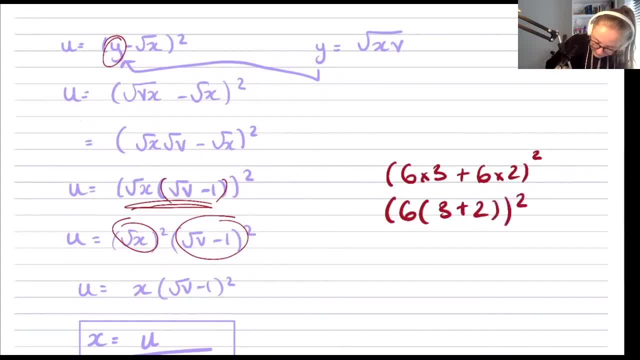 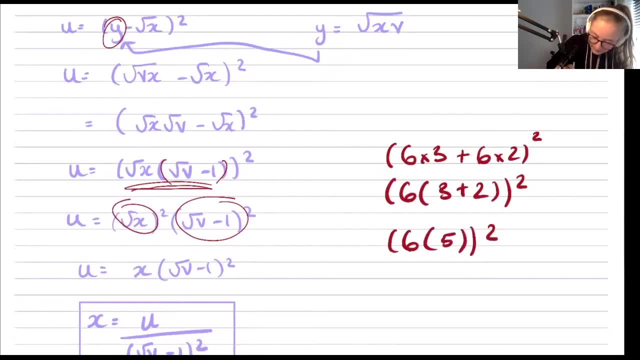 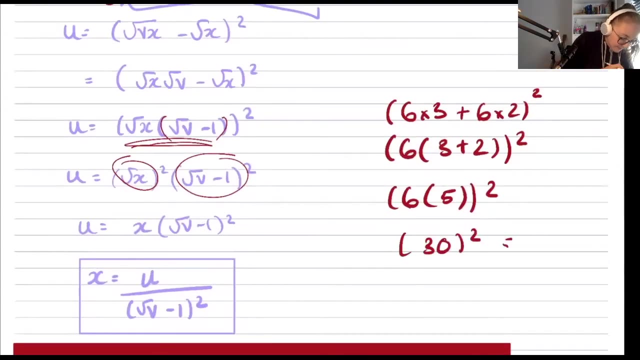 to get this, And then we can go 6 times 2 all squared, 6 times 5 squared, So you can do 30 squared And then 30 squared is equal to 900.. Or instead of doing it this way, we could have done: 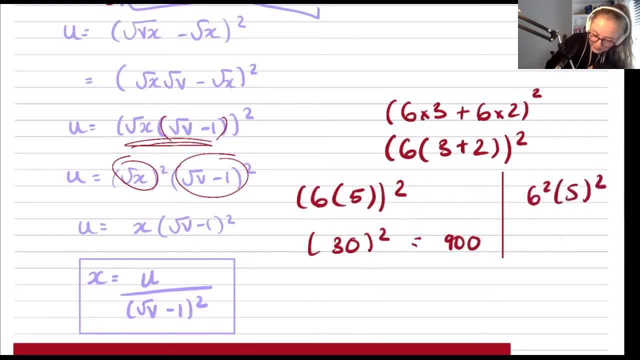 6 squared times 5 squared. So we've pulled that square inside the bracket And we have to square everything inside the bracket So that we have 36 times 25.. And that is also 900.. So if you're not sure about if you're allowed to do something or not, 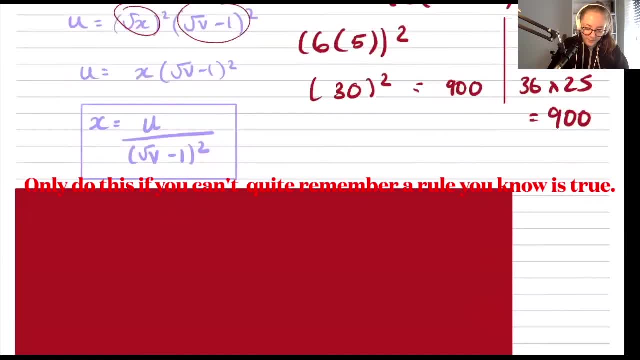 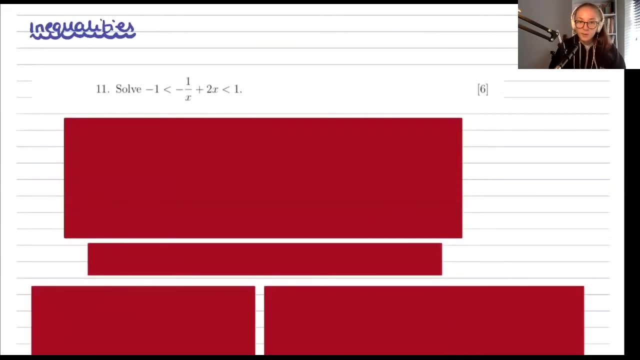 just try it with numbers first and see if it matches up. Okay, our next topic is inequalities. I feel like these questions are quite common in the path And they're really easy to ask, but they're also very, very hard to answer. So I'm going to give you a hand. 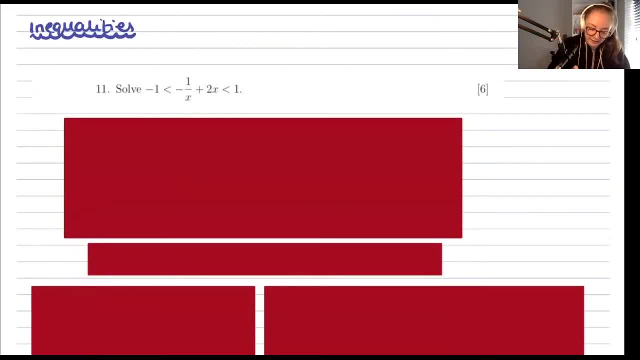 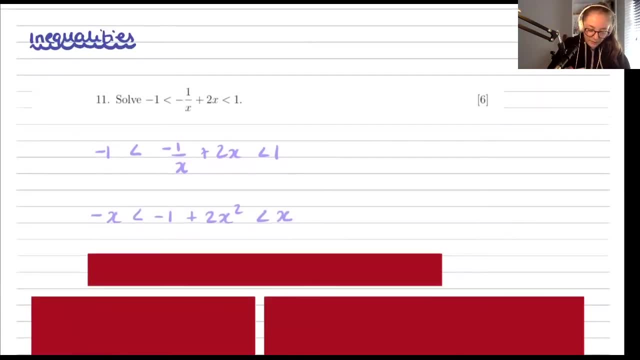 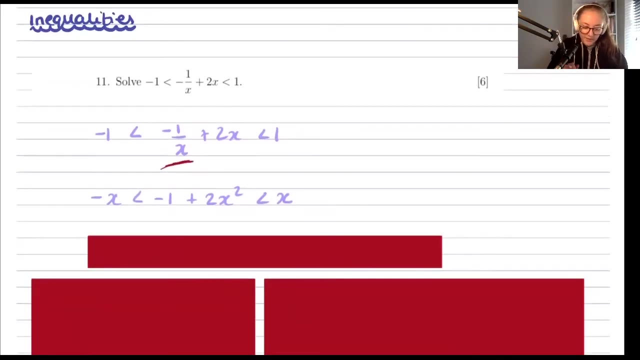 easy to get your head in knots over, so I think the easiest thing to do is to just try and keep the question as clear as possible. so for me, I didn't like having something on the bottom of a fraction. I didn't like having an x on the bottom, so I multiplied everything by x before I started. 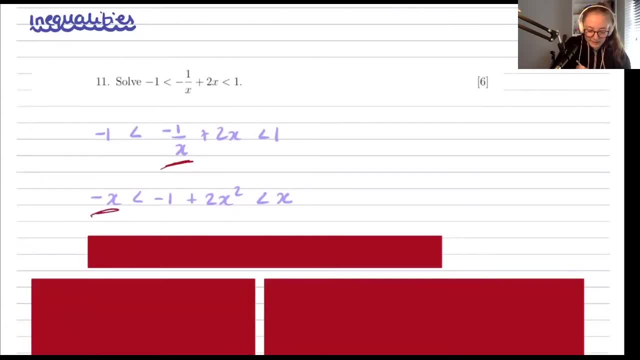 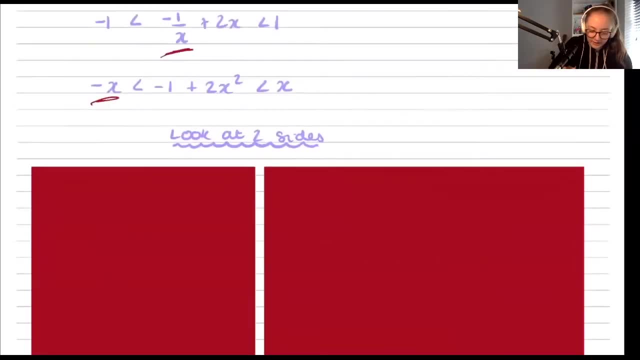 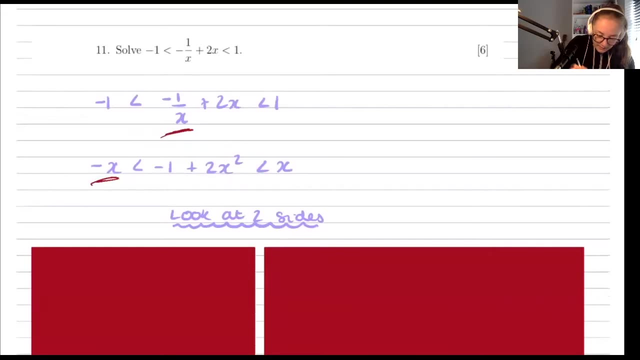 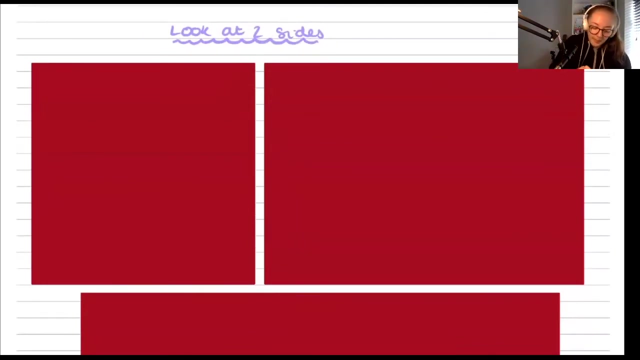 to get: minus x is less than minus 1. plus 2x squared is less than x, and then what we need to do is we need to look at the two sides individually, our two sides being this side and this side, because we're essentially given two bits of information. so I will look at the left first. 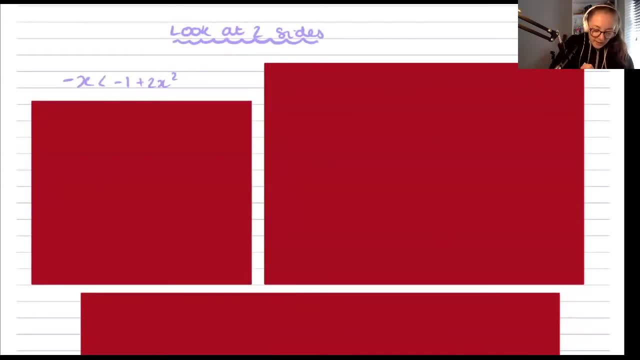 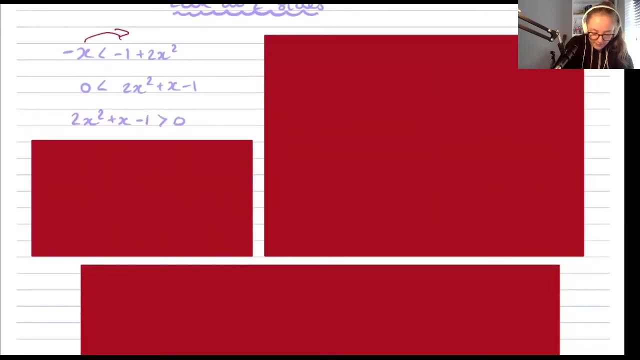 and what this tells us is that you minus x is less than minus 1, plus 2x squared. so I'll rearrange this a little bit, so I move this over to the other side to get 2x squared: plus x minus 1 is greater than zero. and then I don't. 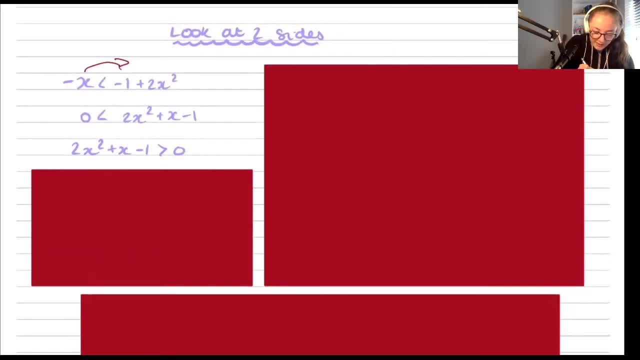 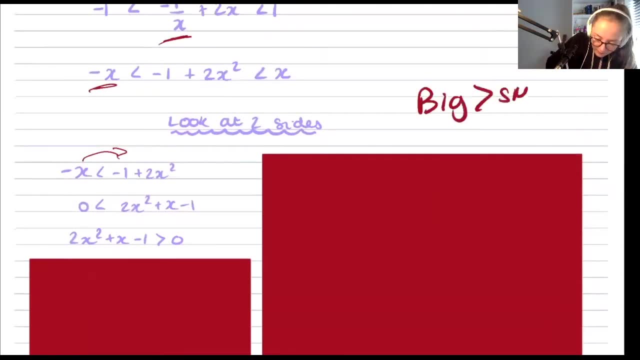 like having the zero on the left hand side, so making sure to keep the statement the same. so if I'm saying big is greater than small, it's the same to say small is less than install big. so all I have to do is get the x squared plus 1x squared plus this. 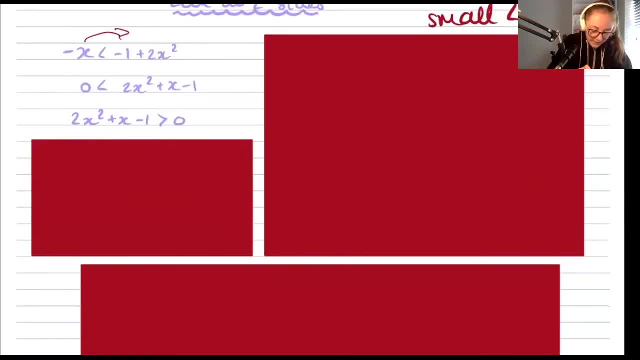 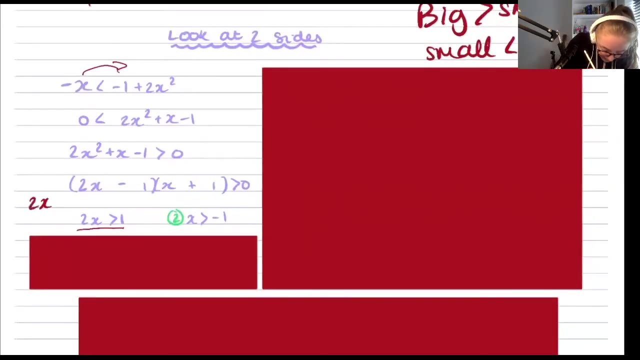 much better. so this pizza piece I've just looked at, how is the other one number equal to 2x to the smaller one gave it? so I just have to go over this, for example, so we can say the swing man is kinds of is the exact opposite of 2x or 2x. all that is. and that's also a cm, but they're actually东, so that's a cm. plus 1x is greater than 0and just because one, x and 1 are even things as a, and then I'm going to factorise this to get two statements, and what this is telling me is that 2x is greater than 1. 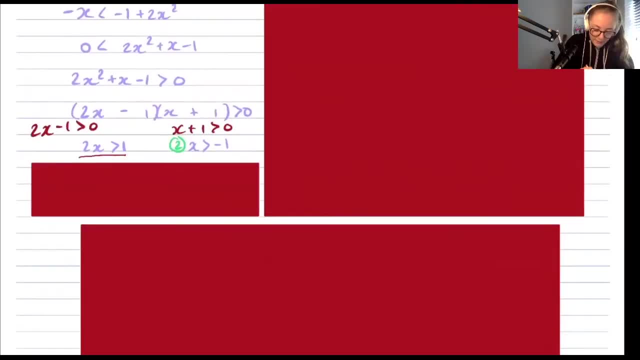 is that you x is greater than 1, because this this came from the fact that 2 x one is greater than 0 and x one is greater a us. So I've rearranged these to get x is greater than a half and x is greater than minus one. Now. 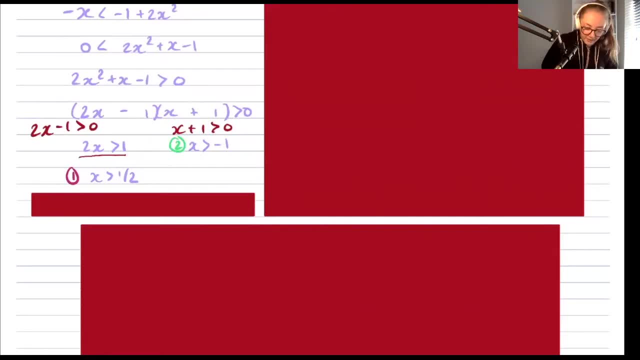 at this point it would be really tempting to say: ah well, if x is greater than minus one and x is greater than a half, then it's not just the same as saying x greater than a half. I would say yes, but we haven't got all of the information yet. So just hold on to that and don't poo-poo any of these. 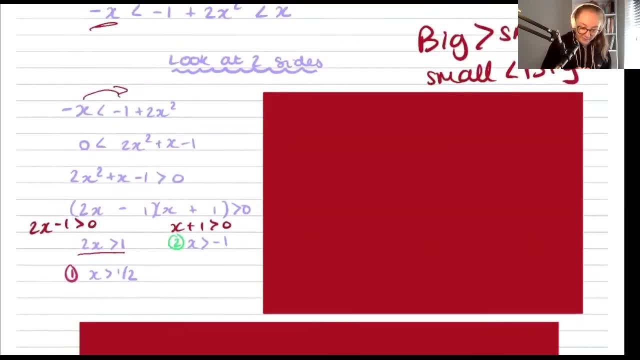 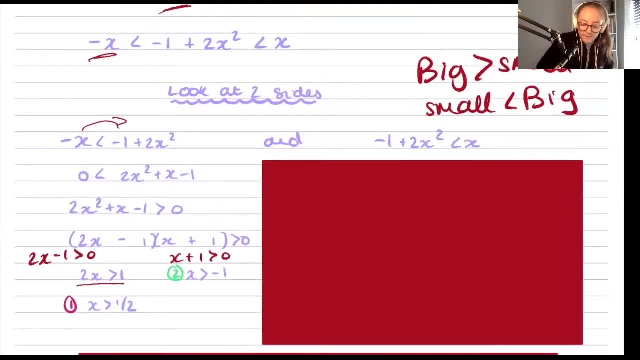 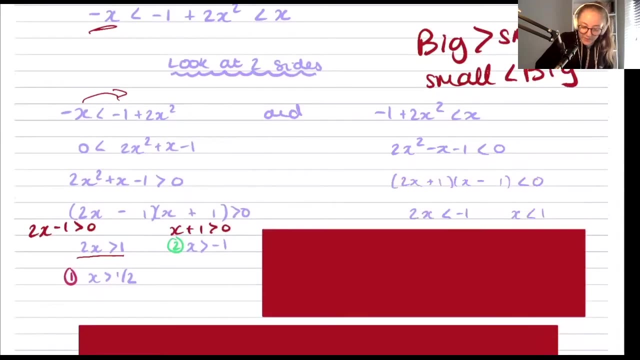 results until you've looked at the other side. So looking at the other side, we have minus one plus two x squared is less than x, and then same jam again. I've rearranged it and factorized it to get this information that two x is less than minus one and x is less than one. 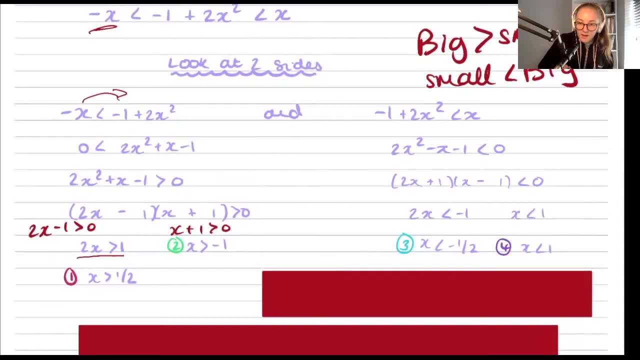 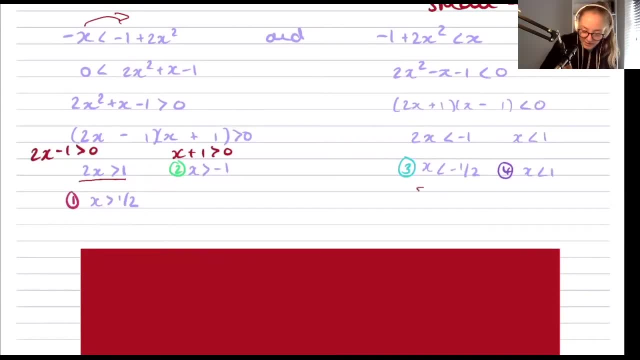 and then x is less than minus a half and x is less than one again. So we are given four bits of information here and again same temptation here to say: oh well, if it's less than one and it's less than minus a half, then it's not just less than minus a. 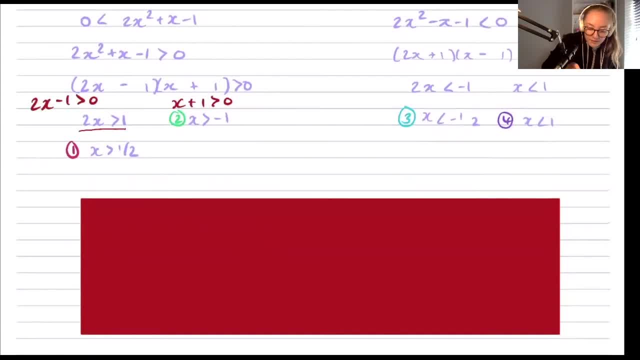 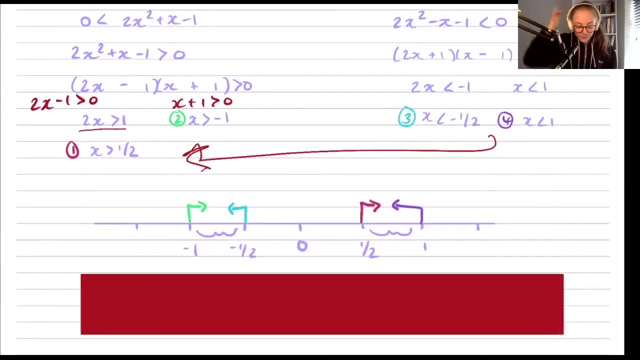 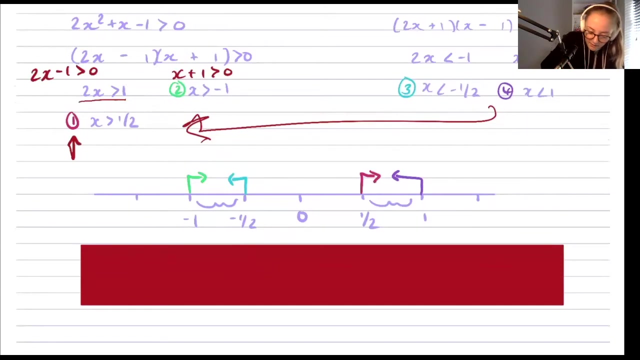 half. Sure, yes, but we also have. we also have this information over here. So the easiest way to interpret what's going on here is to plot a kind of number line to see what we're allowed. So here is a point, number one, I'll call it. I'm saying x is greater than a half, So at half it's got to be. 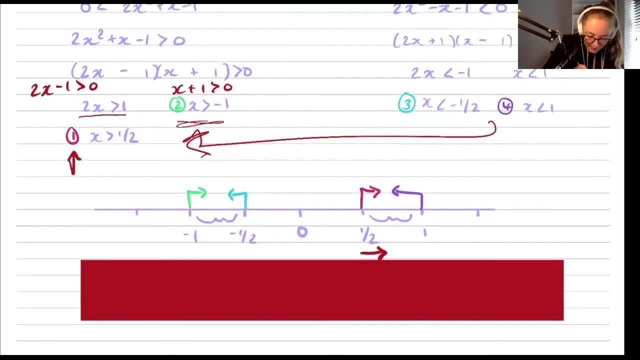 more than that. And then point two here tells us that x is greater than minus one, So down here, x is greater than minus one. Then point three tells us that x is less than minus a half, So down here we can say this. and then point four tells us x is less than 1, so we can say that it's less than that. 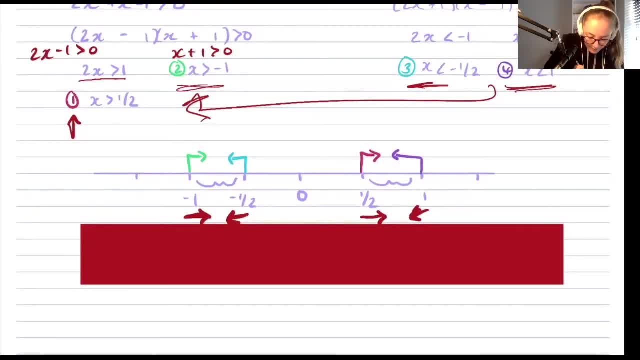 So we can see visually now that it says: well, x can either be between these values or between these values. if we'd kind of taken these, this information here to say the same thing, and if we've taken this information here to say the same thing, we would have missed the fact that we have two ranges. 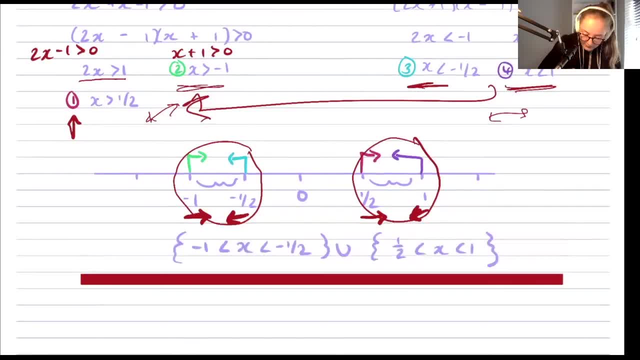 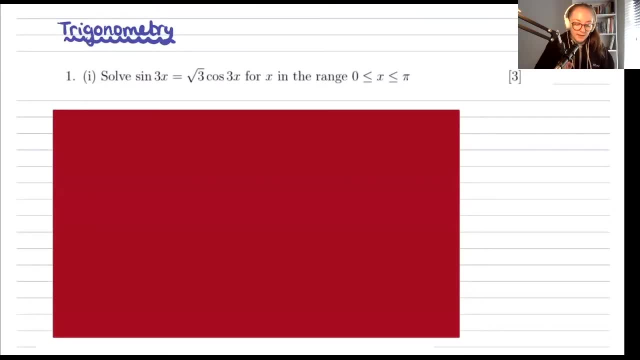 And thus this, this. we can write this in this form where we say that x is between these values or x is between these values. Okay, so next is trigonometry, and we've already used a lot of our trigonometry skills in the geometry section. but this is just kind of pulling out the raw maths and concepts. 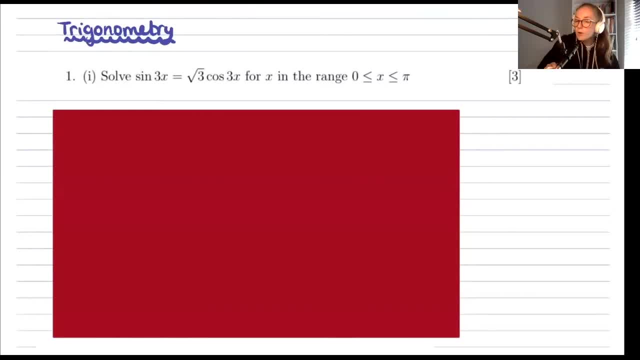 behind trigonometry. This is a question that you've probably had to do in A-level or something similar, but essentially, we are given a trigonometric equation involving signs and causes and we're given a range- be careful to adhere to the range- and we need to find values of x between. 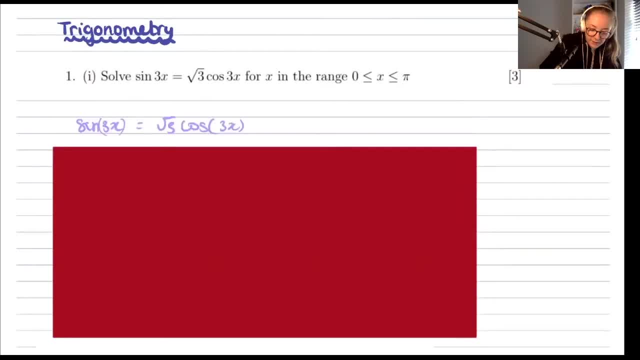 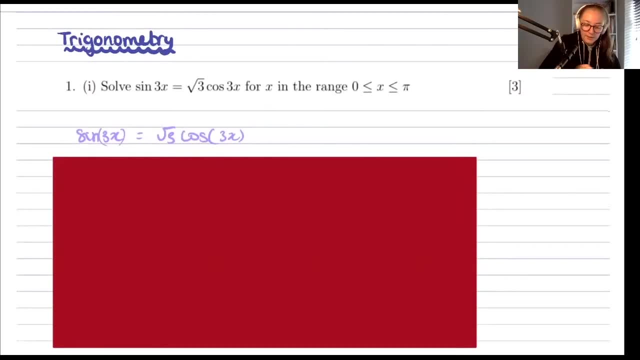 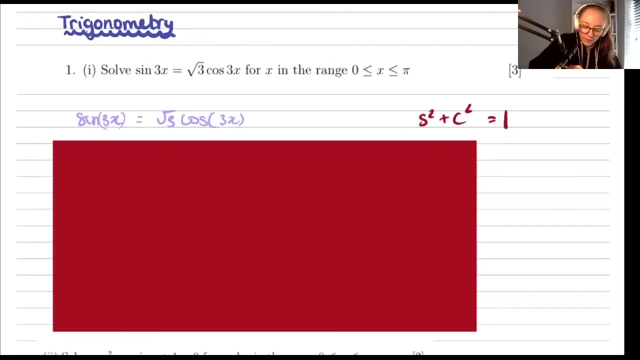 that range. So first things first. I'm just going to write this out again, because I like to write it out again, just to get my head around what's happening and some important information that we know about signs and causes in the relationship is: sine squared plus cos squared equals one, but we're not dealing with sine squareds and cos. 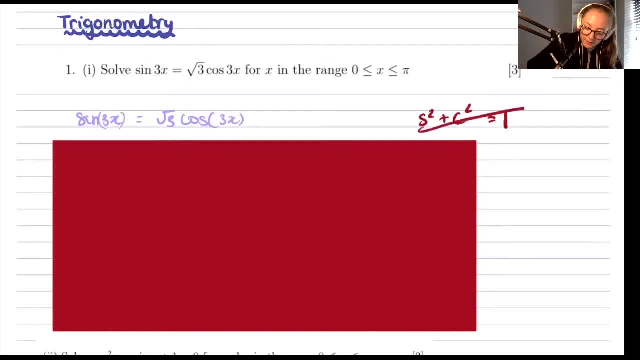 squareds. here we're only dealing with signs and causes, so this is not useful right now. Other bit of useful information that we know is: sine over cos is equal to tan, and this is useful here because we have a sine, we have a cause and we can't relate them without this equation here. 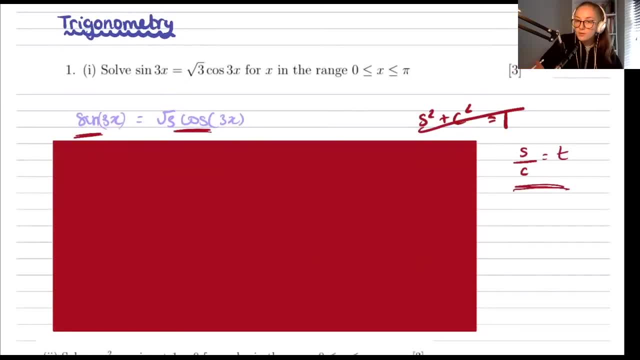 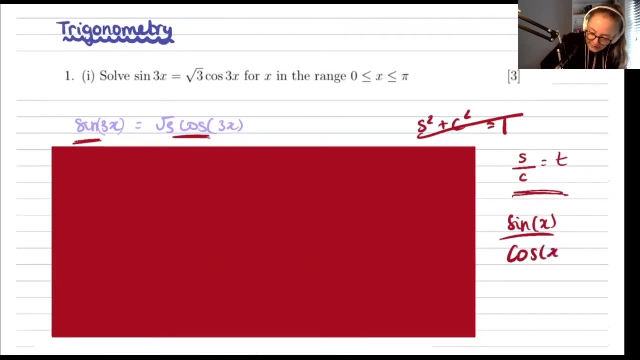 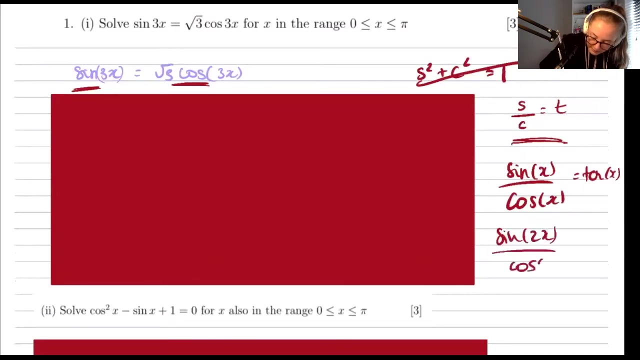 and we, you are just stuck with two different equations that we can't combine. but remember, this is only true if what's this is only true if what's inside the bracket is the same. we can't say, for example, oh, sine 2x over cos x is tan x. that's not true. Luckily for us, they've both got the. 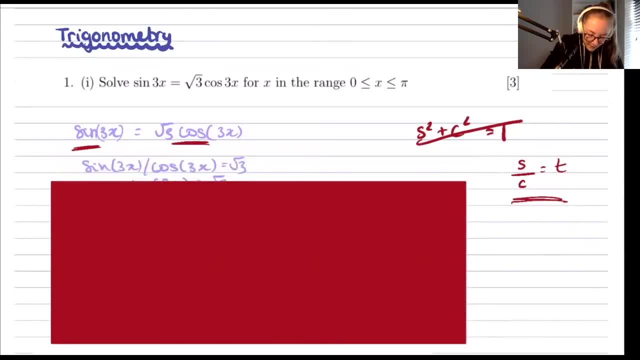 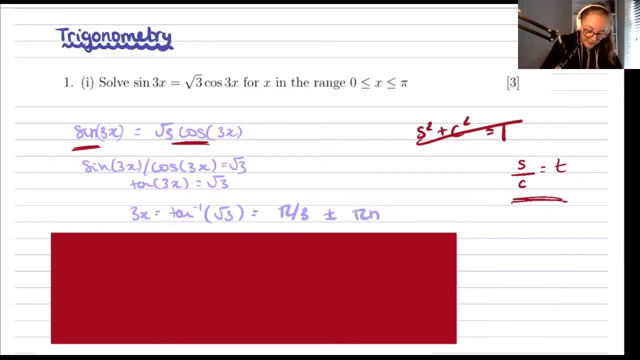 same thing inside the bracket 3x. so we can take the cos underneath the sine and say that tan 3x is root 3, which, if we take the inverse tan, we can see that 3x is equal to pi over 3.. Now at this point it 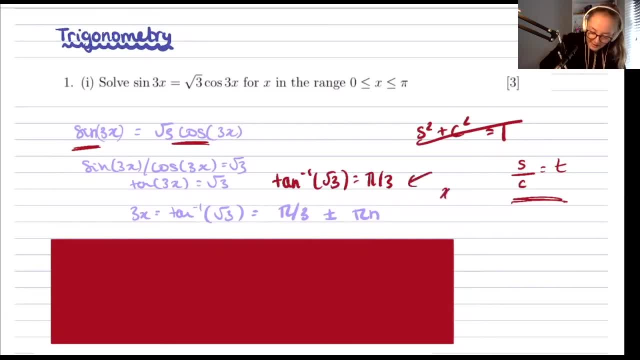 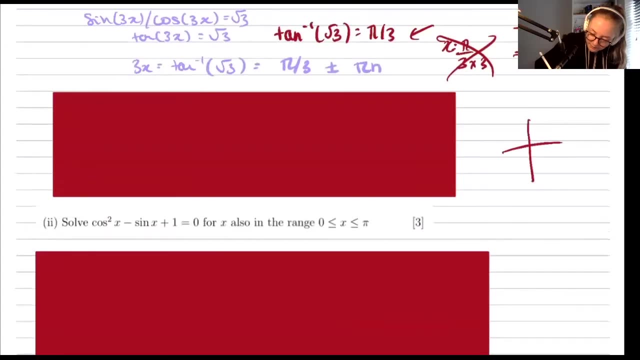 would be really tempting to just divide all of this by 3 to get. x is pi over 3 times 3. but this is not what we should do here, because, um, when we have a tan, we're going to be able to divide all of the tan function. we don't just have that tan function itself, but we have a load of them in a. 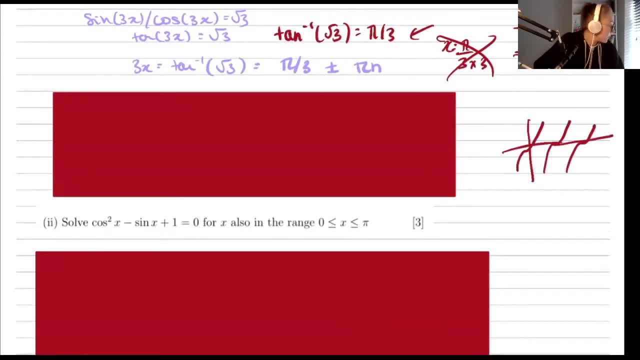 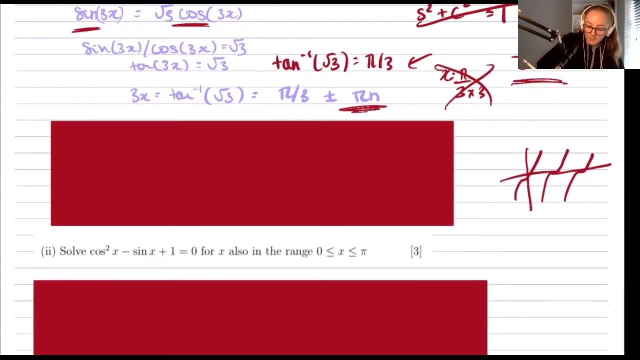 series like this. so when we divide um- so I've added in this spacing here, I suppose, which says um, that from minus infinity to infinity, if you will, um our tan minus 1 over root 3 is pi over 3 plus or minus pi n. but when we divide by this 3 we don't. 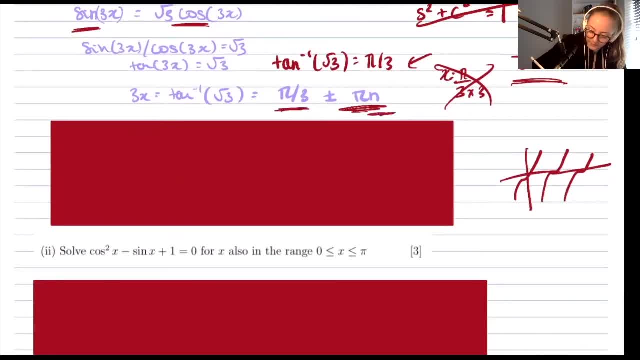 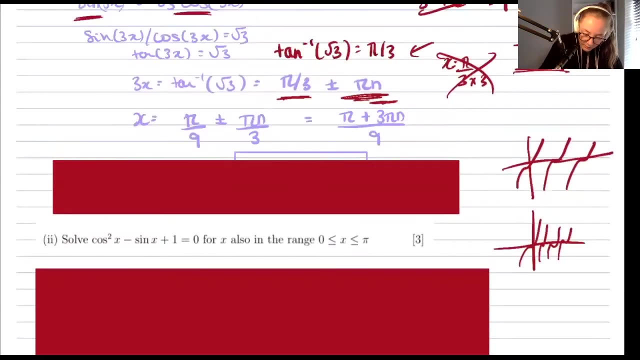 just decrease this, we also decrease the spacing as well. so it would be kind of more like this: so you need to be careful that you don't divide too early, otherwise you will not shrink down the spacing as well, and then, once you've done that, you just decide the ends that keep. 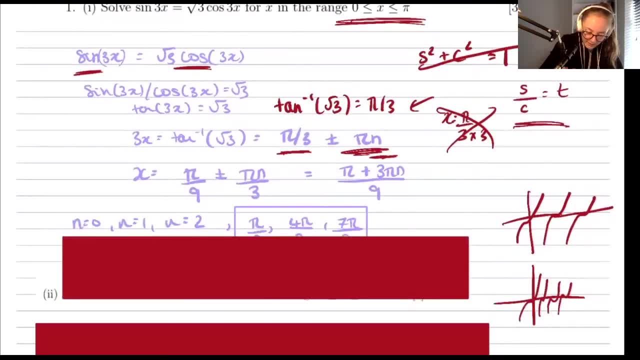 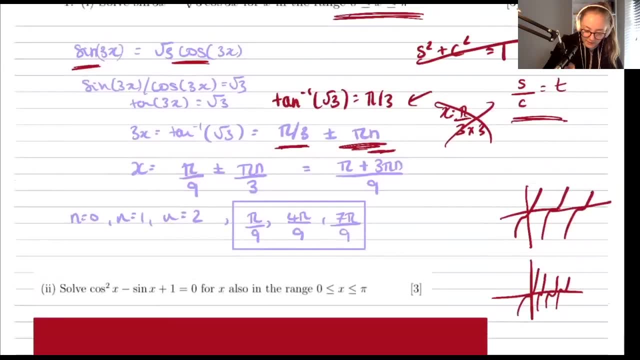 the x value within these range. so for this one it um worked when n was 0, n was 1 and n was 2 and we get three values. if we use n is 3, then it'll become larger than pi, and if we use n is minus. 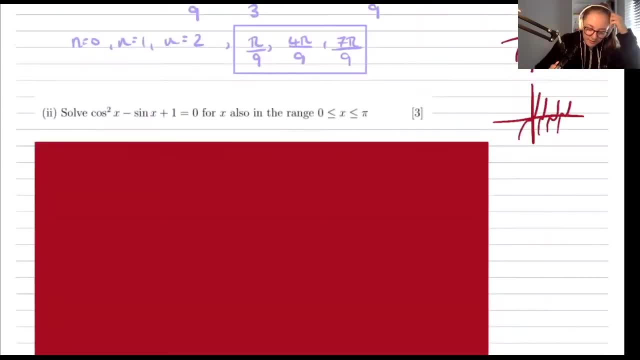 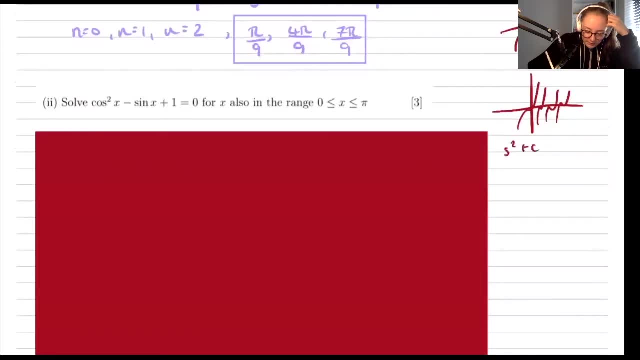 1, then it'll be less than 0.. Okay, so the second part. if we think about our equations again, then we have sine squared plus cos squared is 1 and we have sine over cos is tan. Well, for this one we have a cos squared, a sine, a 1 and a 0. So there is no way of relating cos squared. 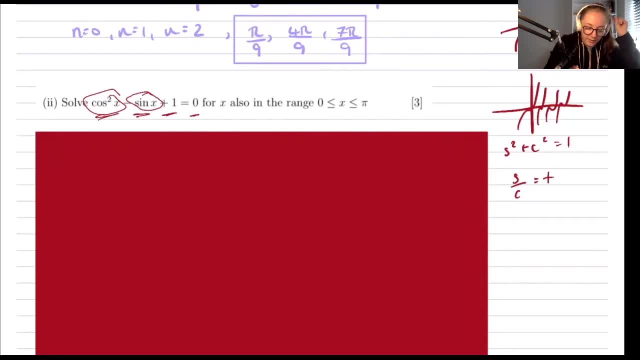 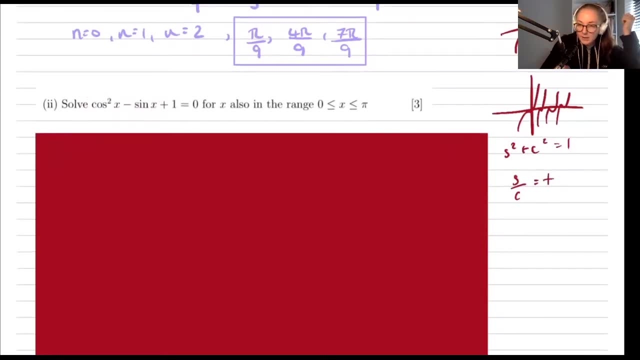 and just sine on its own. All we can do is replace one of these terms to come up with the relationship that we can work with. So the best way of doing this is to replace this cos squared with a this uh, 1 minus sine squared. 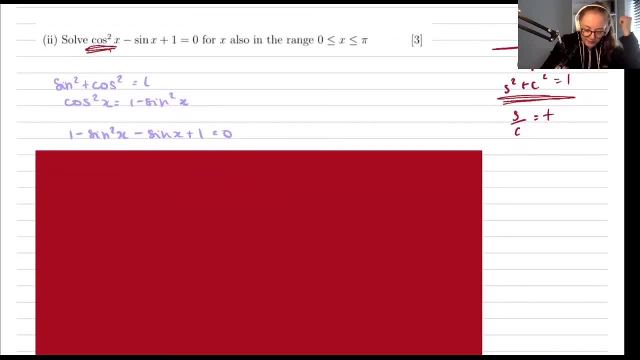 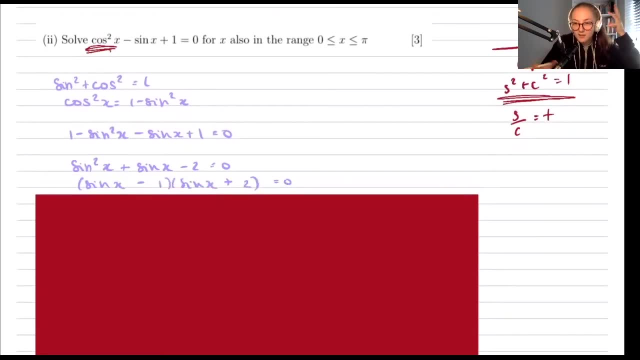 like so, And right now that doesn't really look any less complicated, uh, but it does mean that we can factorize this. So if we just imagine that sine x is just y or something, so if we say sine x is y, then what are we going to do? 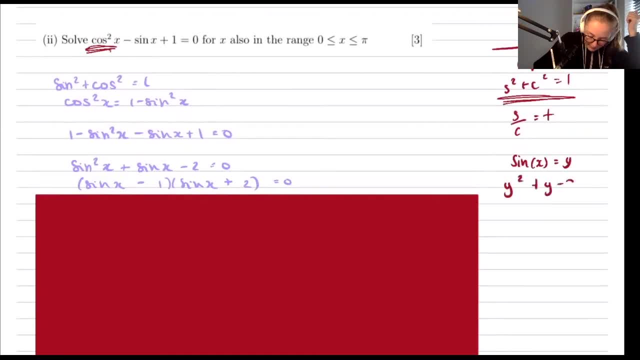 So what our equation will look like is y squared plus y minus 2, and we know how to factorize that, don't we Easy. And then we can just stick our sine x back in. So if you're a bit confused about factorizing, 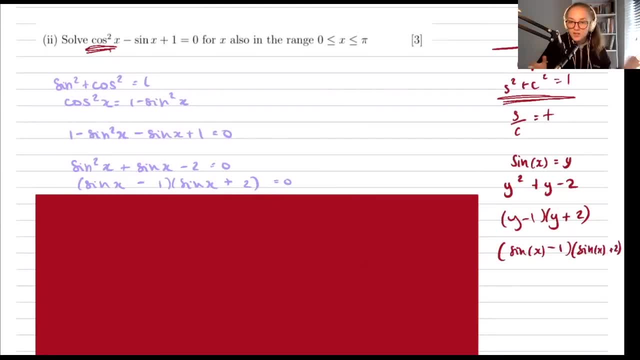 signs or causes or any other more complex terms. just call it something else. first Work, factorize that something else and then stick it back in at the end And it'll help you out. It'll help you use confusion- same thing as if you try and factorize something like this: 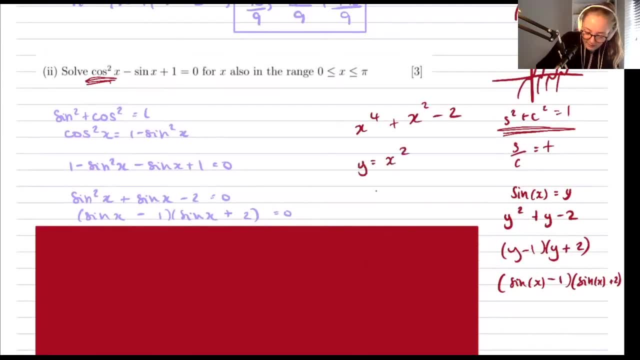 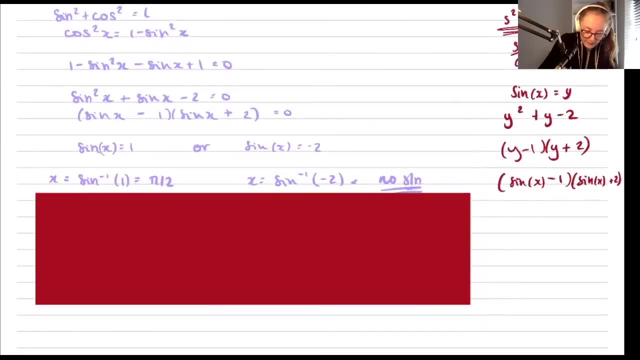 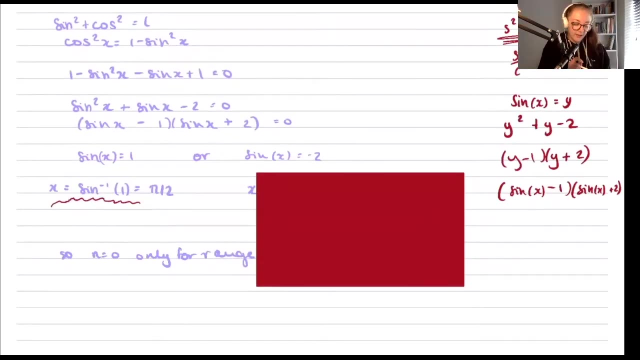 it's much easier to just say: oh well, y is x squared, So we have y squared plus y minus 2, and that's much easier to factorize again. So that gives us two equations: We have sine x is equal to 1 and we have sine x equal to minus 2.. We get x is the inverse sine of1, which is pi over 2, and 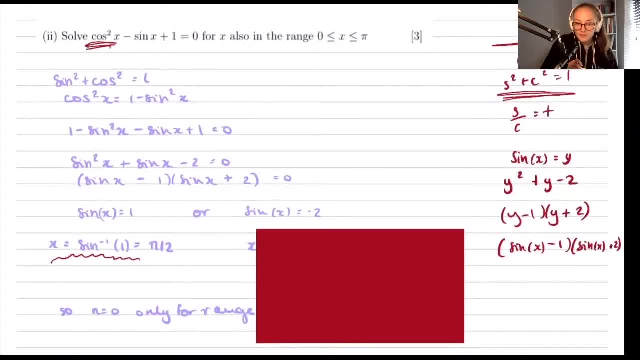 then if we think about how often that will repeat itself in a sine function, um, then we'll see between naught and pi it's not going to repeat itself again. so within the range pi over 2 is our only answer. and then if we take the inverse sine of, 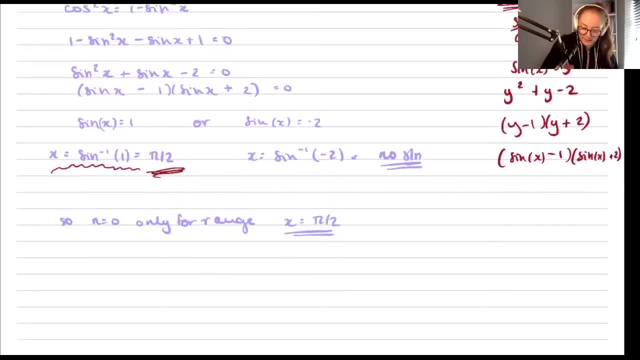 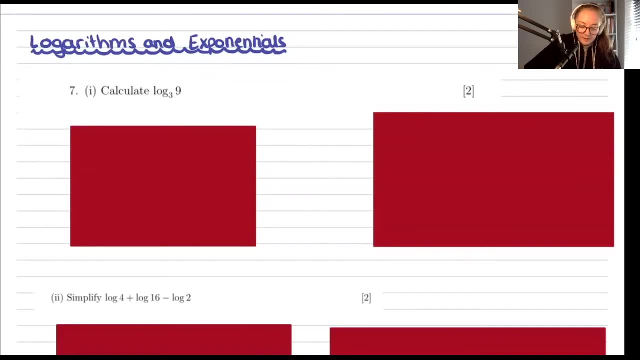 minus 2, we don't get the solution. so our answer is just pi over 2, okay, so moving on. uh, we'll look at logs and exponentials now. this question, this first question, is a bit of a dream, um, but it just requires you to remember what a log is telling you. so a log: so x equals. i've just called our. 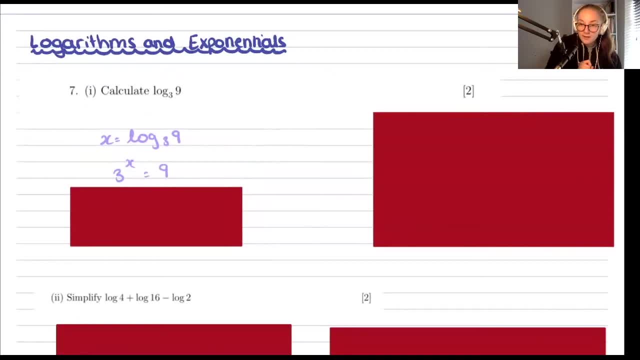 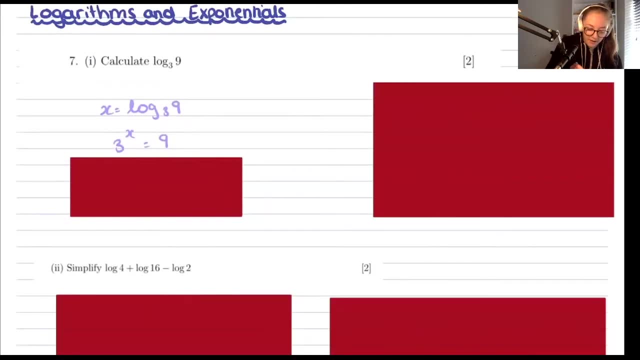 output x. so log 3 of 9 um is the same as saying that 3 to the power of our answer. so i've called that x is equal to 9. so what x would give us 9? x is 2. i have kind of a verbal way of remembering. 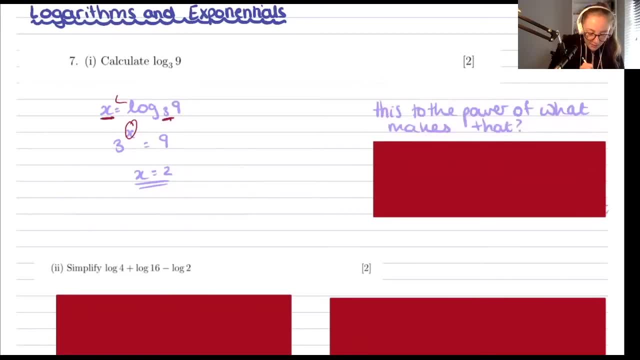 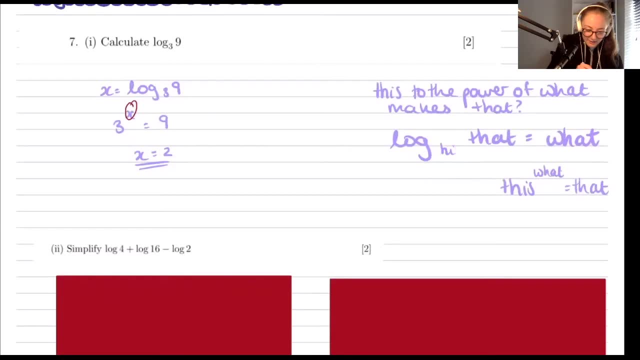 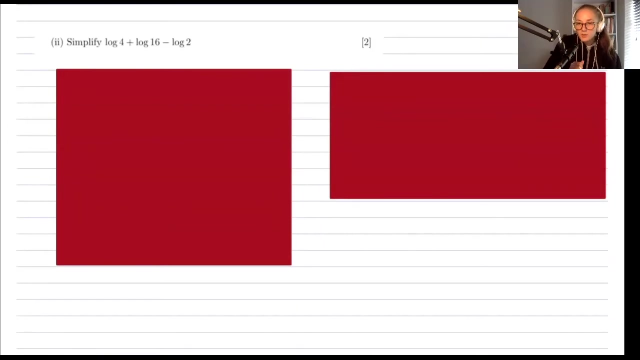 what logs mean. i say this to the power of what makes that. you can see, i've, i've written it in words here: so this, so this, the power of what makes that, and then the what is what we want to know in this case. okay, this next part is just about, uh, combining logarithms, which i'm sure you all already know. 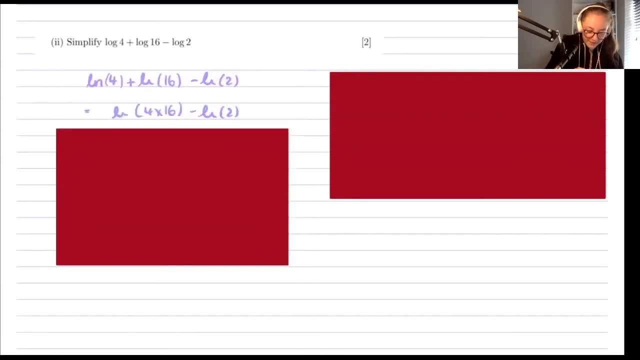 the rules for this, but, um, if we're adding natural logs, then we can multiply inside the bracket, and if we are minusing a natural log, then we can divide inside the bracket. and that is just all you need to do. and if you're really smart, you probably have noticed. 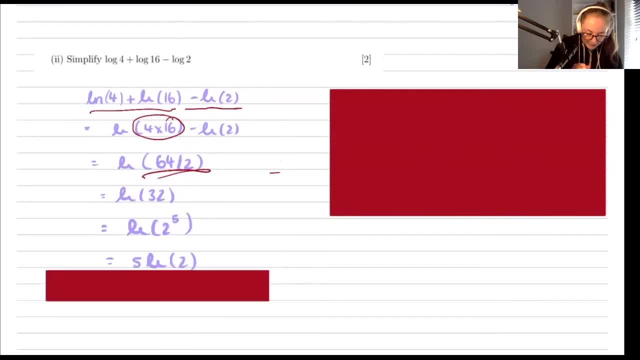 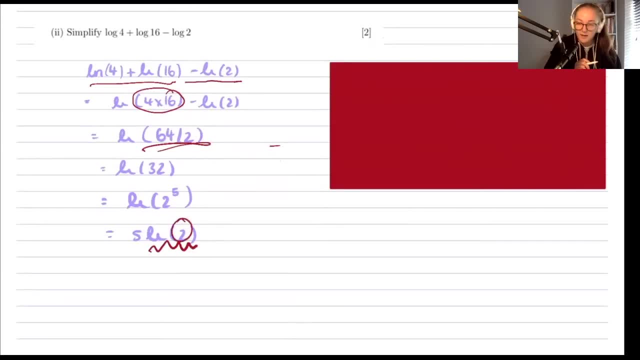 that 32 is the same as 2 to the power of 5. so we can simplify this again to get the smallest internal uh number in this log as we can. so we can get 5 ln 2 or a different way of working this out. 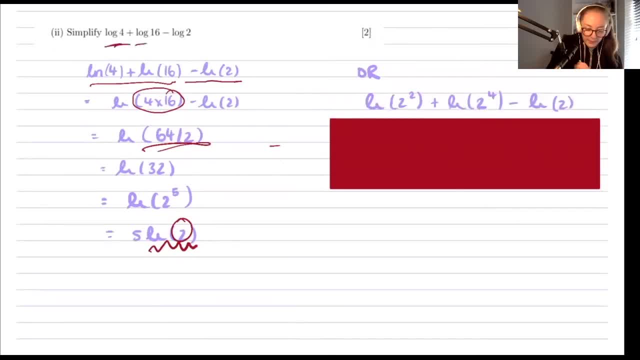 is to notice that 4 is 2 squared 16 is 2 to the power of 4 and 2 is 2 to the power of 1 um. and then we can use the rule where we take the powers down to just add these logarithms up and get 5 ln 2 immediately. 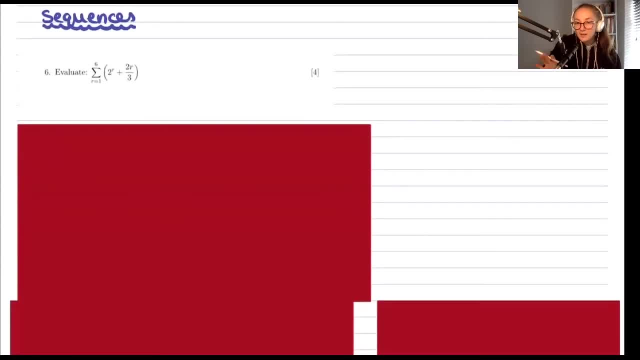 now sequences. some people take these really naturally and other people don't. um, i'm probably one of the ones again who takes this less naturally. um, but it's all about spotting patterns. so in a question like this, um, we are not required to spot a pattern, we are just tested on whether 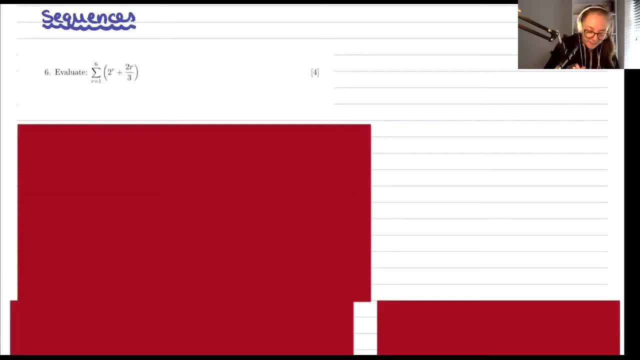 we know how to handle arithmetic and geometric series. so what this is telling us- if you're not familiar with the sum sign- is we want to um add values of this, taking our first value when r is 1 and then ending when r is 6.. so, if that didn't make sense, what we're essentially 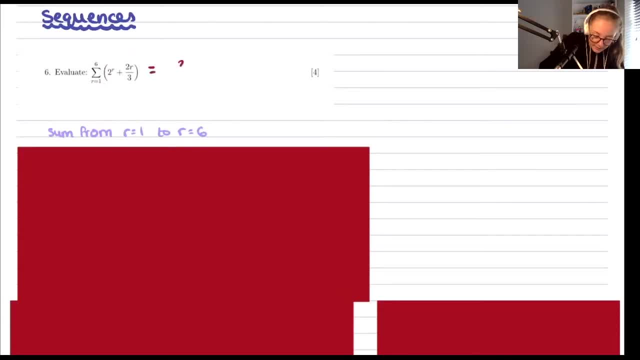 doing is we're saying our sum is 2 to the power of 1 plus 2 times 1 over 3 plus 2 to the power of 2 plus 2 times 2 over 3 plus 2 to the power of 3 plus 2 times 3 over 3, and so on all the way up to 6. 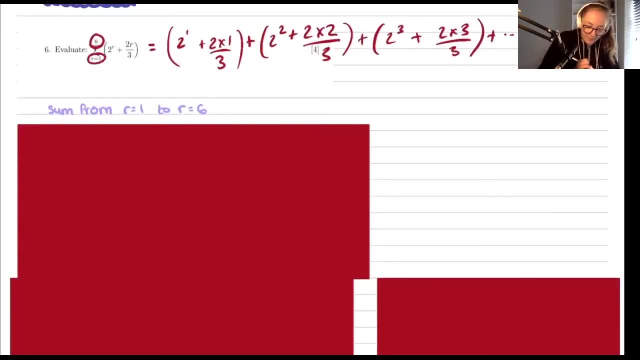 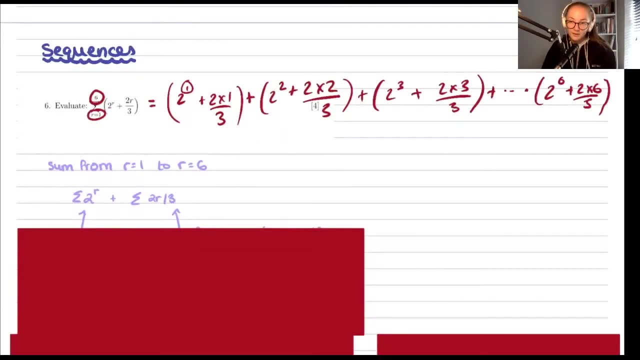 because 6 is our sum top number and 1 is our bottom number. so we start at 1 and we end at 6, but a better way to handle this would be to split our sum up. so the best way i can describe splitting up the sum 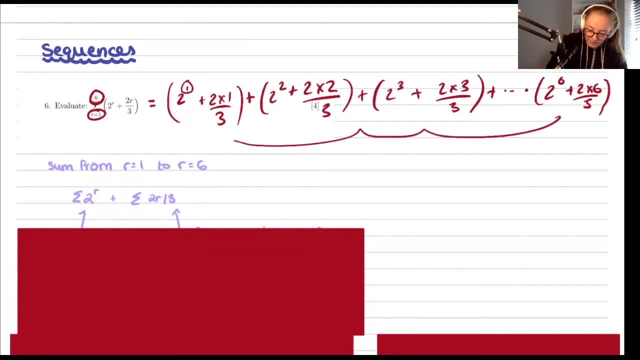 is well, since we're saying this is true, right. well, this is no different from saying, if we rearrange this, 2 to the power of 1 plus 2, to the power of 2 plus 2, to the power of 3 plus 2, to the power of: 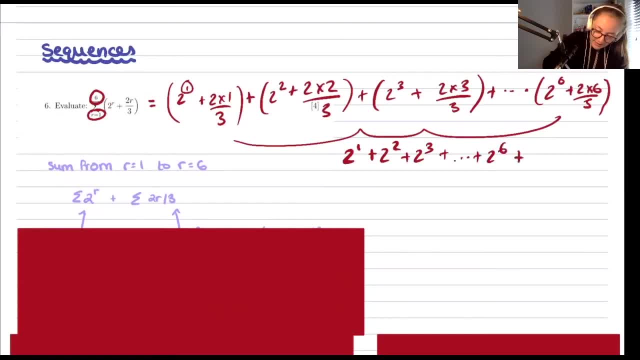 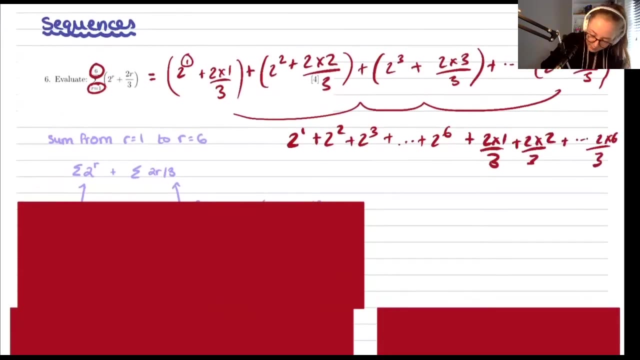 plus plus 2 to the power of 6, and then add that on to 2 times 1 over 3, plus 2 times 2 over 3, plus 2 times 6 over 3.. and essentially what we've done is we've changed the sum to say to the sum 2 to the power of r from 1 to 6 plus sum2r over 3. 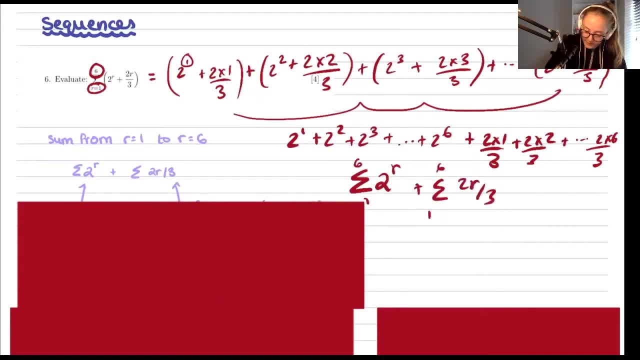 to r, from 1 to 6, plus sum 2r over 3 from 1 to 6, plus sum2r over 3, from 1 to 6, plus 2r over 3 from snacking 1.. from one to six, and then we can also factorize this two over three over here. 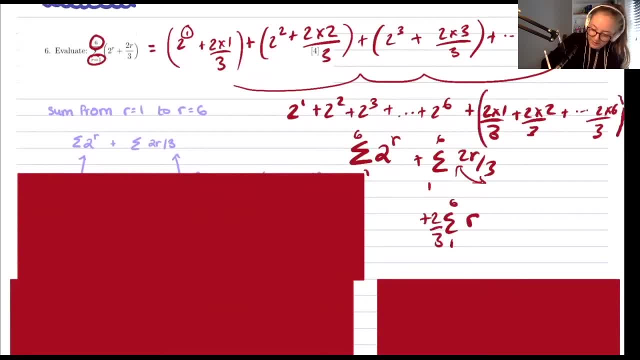 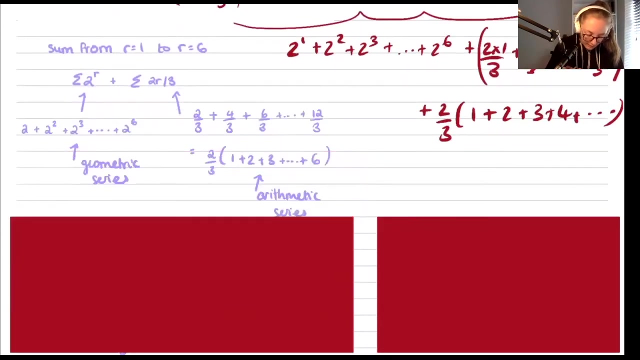 like this, because if you see, we look at all of these over here, we- that is the same as saying so, i'll just get rid of all this mess. that is the same as saying so on. so, bearing all that in mind, we see that we have two series, we have a geometric series and we have 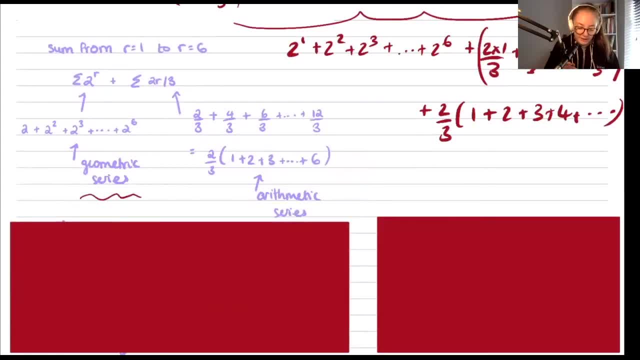 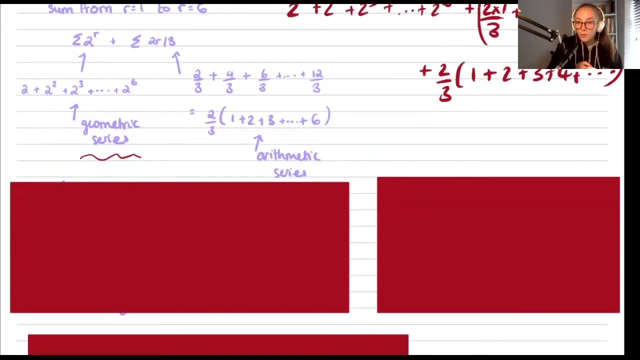 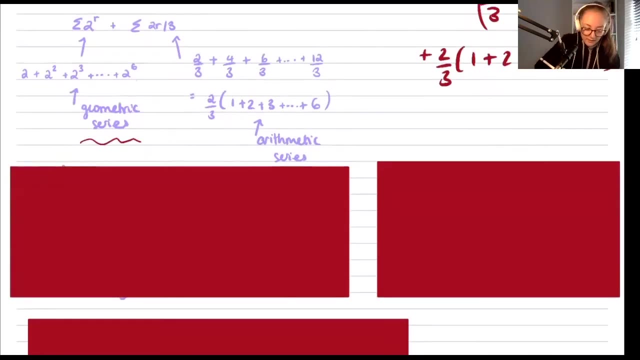 an arithmetic series, and if you're not too sure what these are, um, so you've not done them in school yet. essentially, a geometric series is one where you um multiply your terms by something each time time, So you could have one as your first term and then our next term say: we want to multiply. 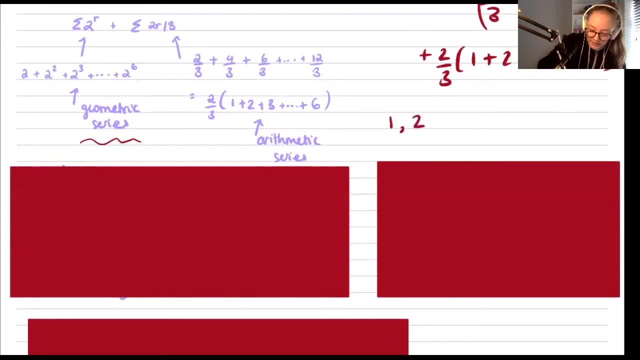 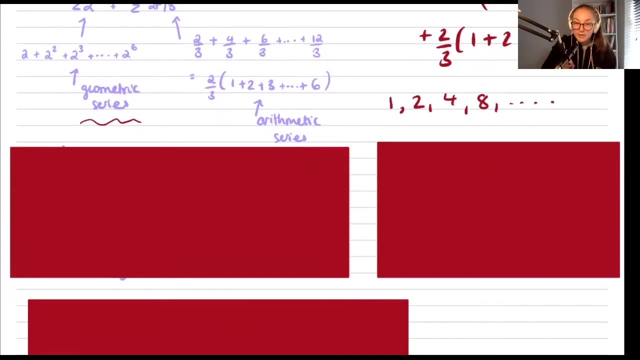 by two every time, then we'd have one, the second term would be two. the second term would be two times two, which is four. the second term two times two times two, so four times two, so eight, and so on. That's our progression. And then an arithmetic series is one where we add something. 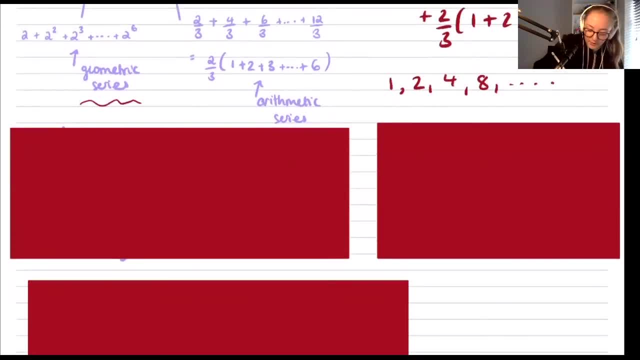 on each time or take something away each time. So, for example, if we say our first term is one, then an example for an arithmetic series would be if we add three each time, So you could have one, and then add three to one and we have four, and add three to four and we have seven. 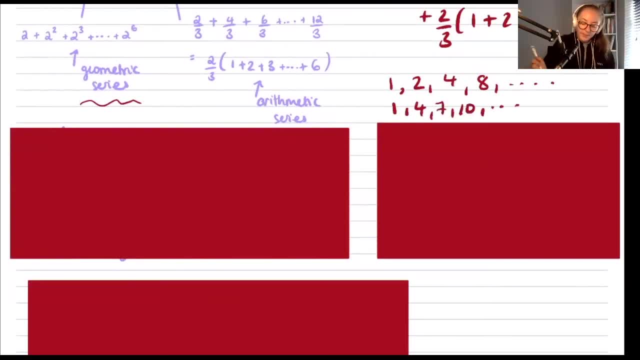 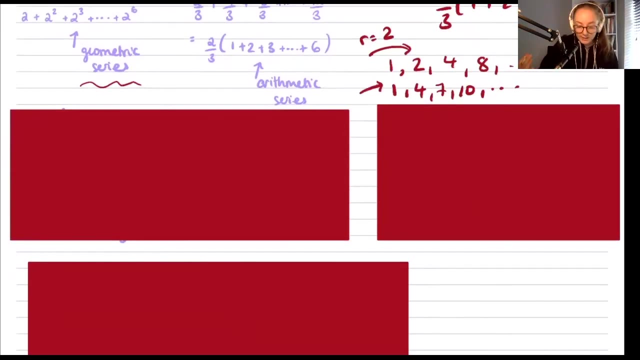 add three to seven, we have 10, and so on. And so for this equation here, what we did was we times by two every time. So we would say that our common ratio, or r, is two, And for this one we would say that the spacing between each term 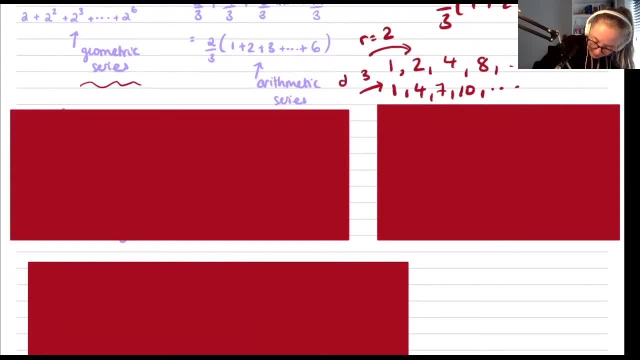 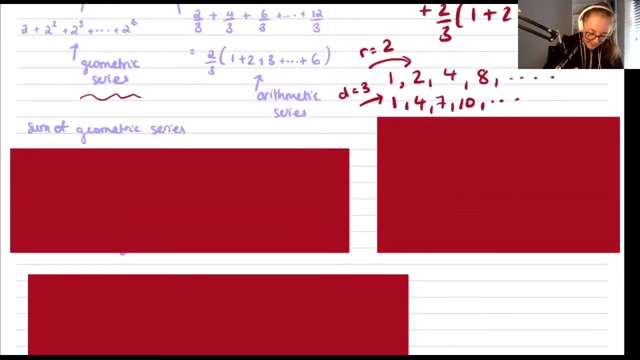 is three, and we can call that d for difference, So we'll have to bear that in mind. Now there are some equations that you will learn in school, and you will learn their proofs in school as well, if you haven't already. But for now, you're just going to have to memorize them. But in order to find the 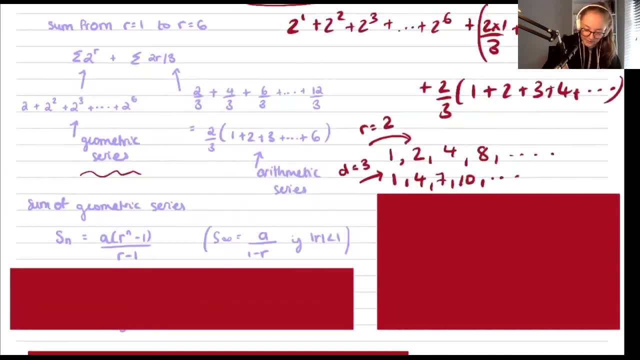 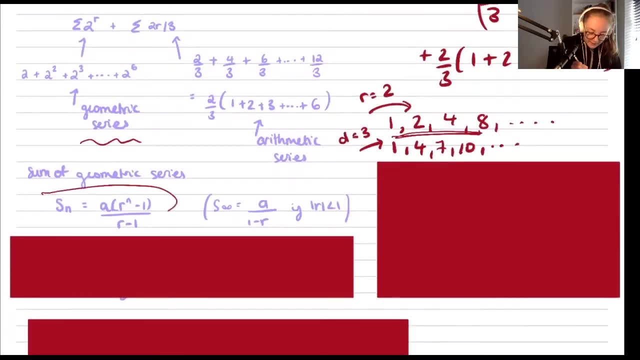 sum of the terms. we're going to have to memorize them. So we're going to have to memorize them of a geometric series. So our geometric series being this first one here, So that would be one plus two plus four plus eight, and so on, We have this nifty little equation which says the sum to 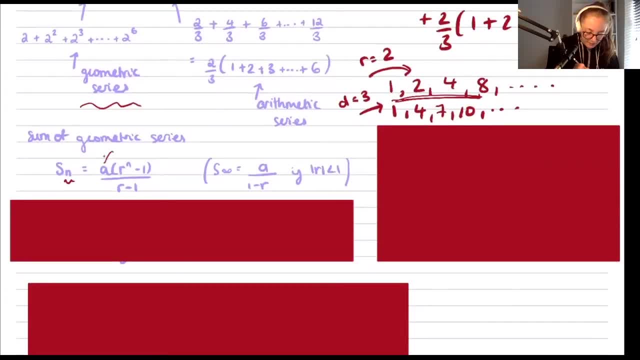 n of this series, our a, which is our first term, multiplied by r, which is our common ratio to the power of n, which is the number that we go up to in our series. So for example here, six minus one- that was in brackets- divided by r, our common ratio minus one. Again, you'll just 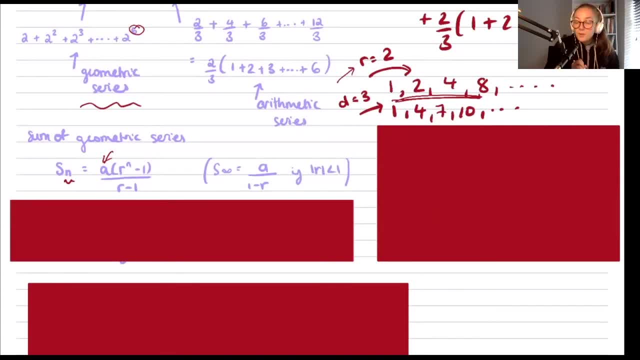 have to trust. that's true right now. But a fun thing we could also do for the geometric series is, rather than going up to a specified value, such as n, we can also sum to infinity if our r is less than one, Because we'll be adding on smaller and smaller things until it just kind of 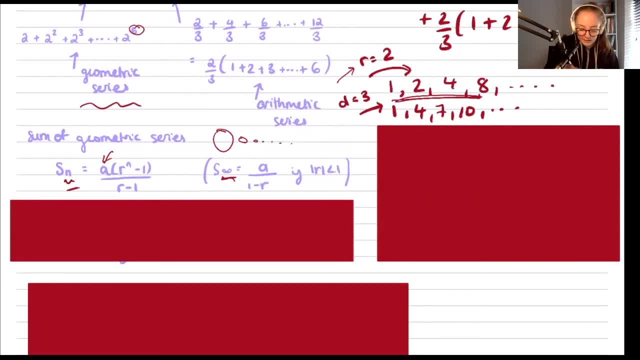 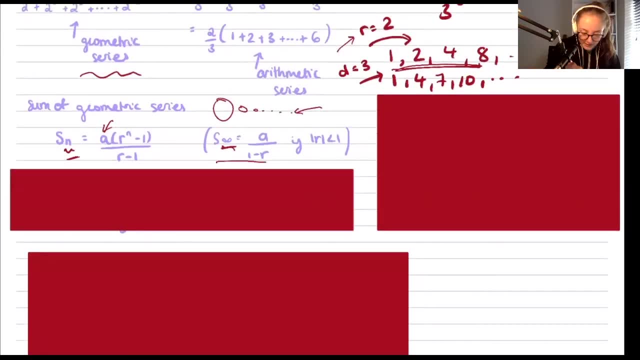 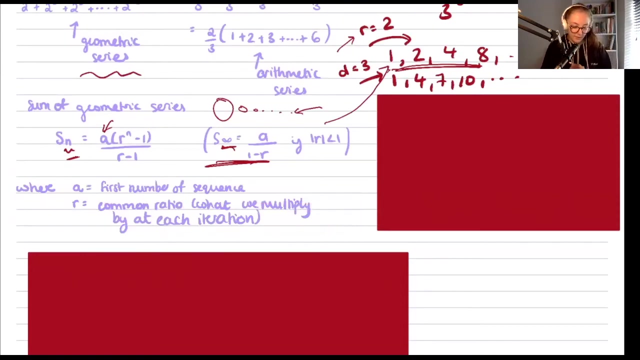 lands Or tends to a value, because this is just the next term- is becoming closer and closer to zero. So an equation for our sum to infinity is a, our first term. So for this progression here it was one divided by one minus r, our common ratio. I've just written a few notes here so that you. 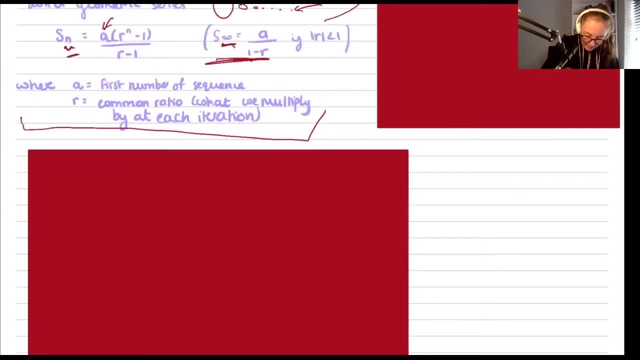 can see and remember what the terms mean. And then our second part is going to be the sum to infinity. So we're going to have to do this. So we're going to have to do this, So we're going to have to do this. 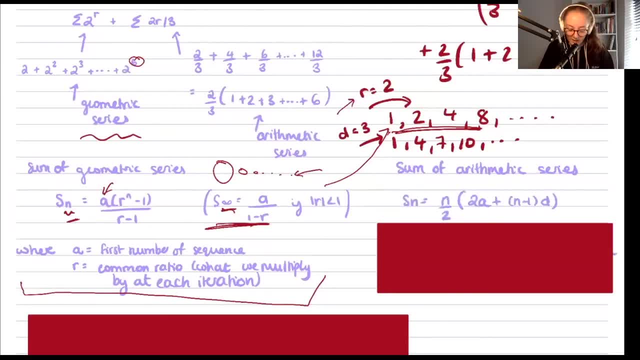 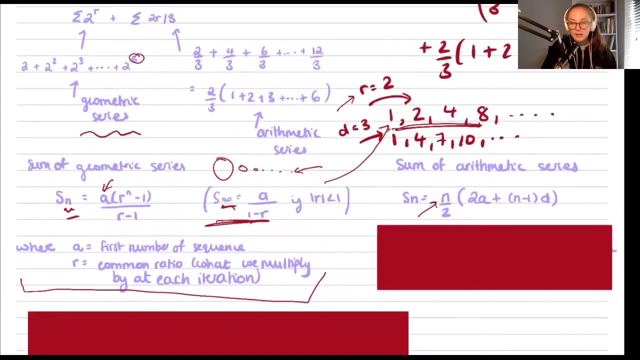 And then later and later on. in the case of an arithmetic series so similar, we have an equation that tell us what the sum to a specific value is: So, n, So here our equation is n. So let's say we're going up to six values. 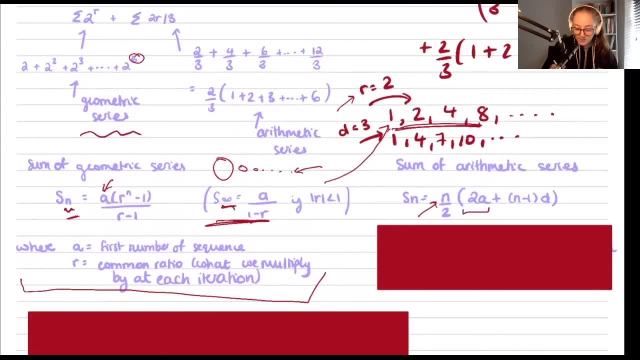 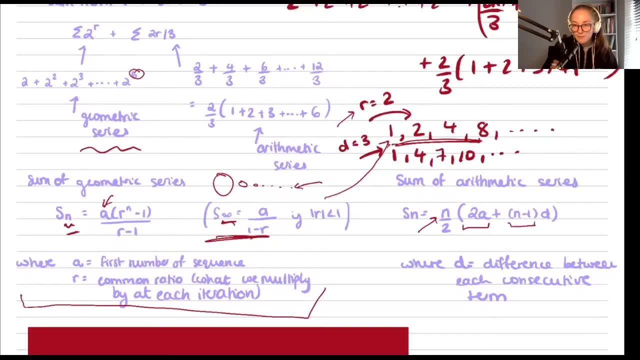 again, N is 6. Divided by 2. Multiplied by 2, a, where a is our first term, And then plus n, minus one. So let's say that was six again. So if you look at the first term, what we're doing is we're. 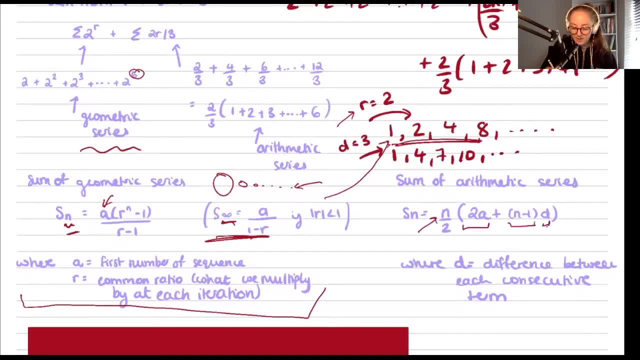 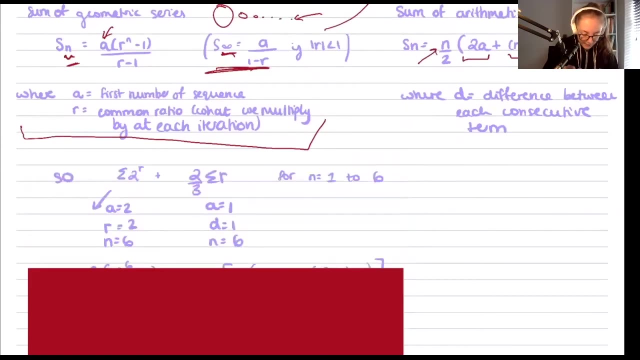 multiplied by d, which is the difference between our terms. so for this little progression here, it was three. so anyway, now we want to apply that to the equations that we have. so what we're looking at here is a geometric series where we start at two and then we multiply by two at each term. 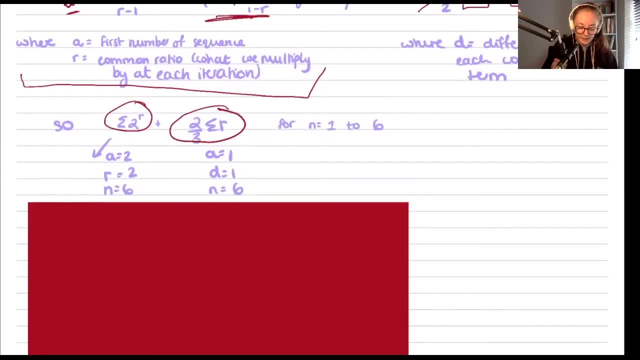 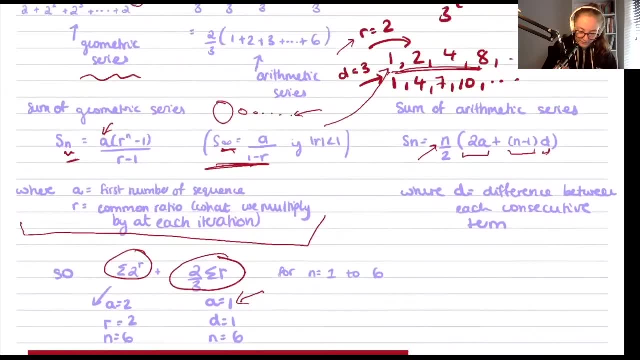 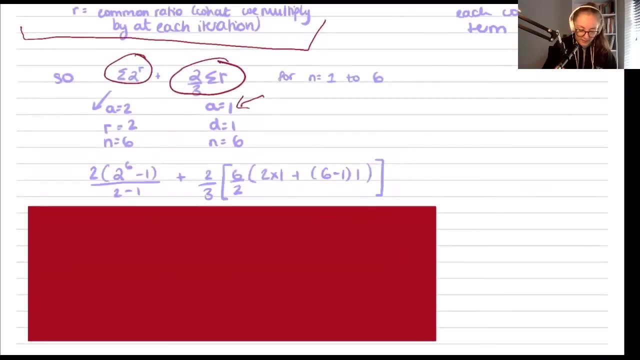 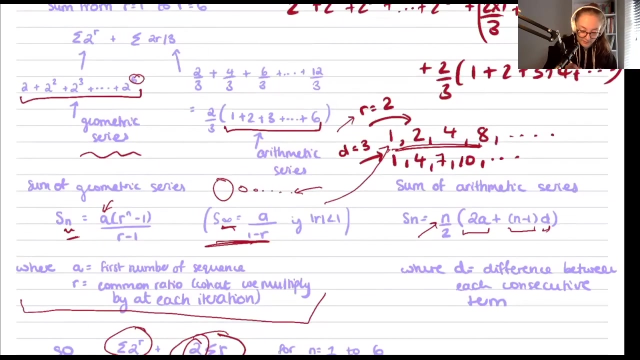 and then what we're looking at here is an arithmetic term where we start at one and we add one each time, as we can see from here. so if we plug these values in, don't forget there's two over three on the outside, because we took that factor out when we came up with this arithmetic. 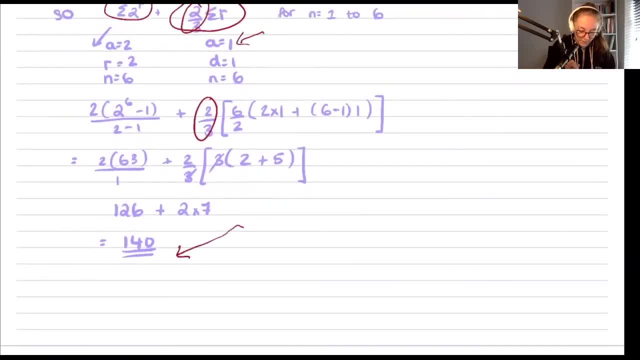 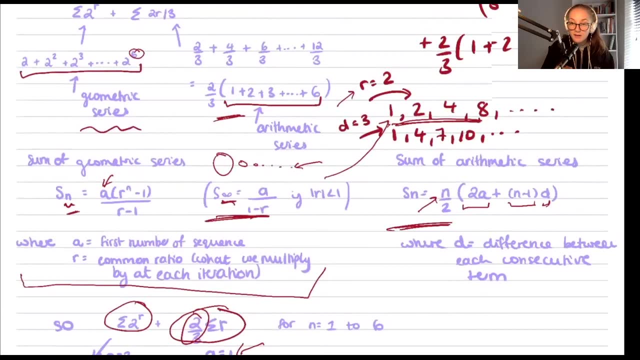 series, we can work this out to get 140.. Now, just as a side note, if you're wondering why there's no sum to infinity for an arithmetic series, that's because the thing that you're adding on each time is not shrinking, it is staying the. 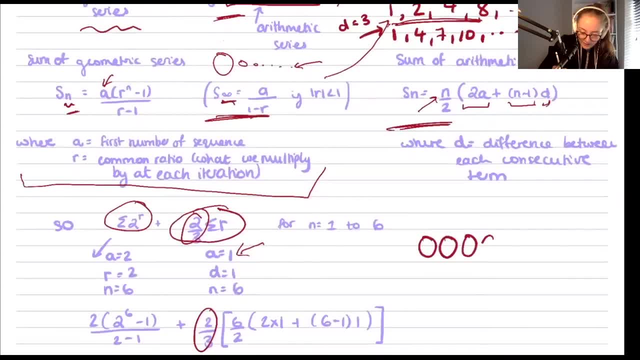 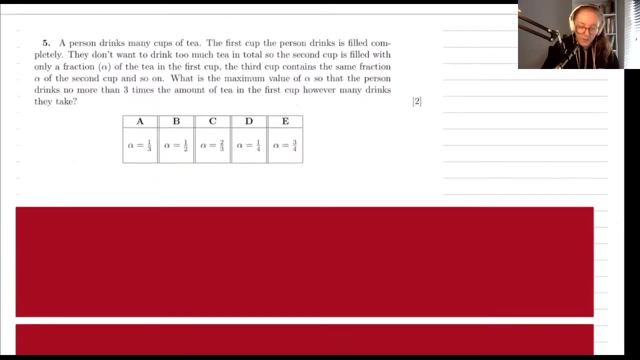 same size. so we're essentially adding lots of things the same size. so as we go to infinity, as we add an infinite amount of these on, we will get an infinite answer. so the sum to infinity of кр collection and as we go up there, we add an infinite number of limits across all three parts. 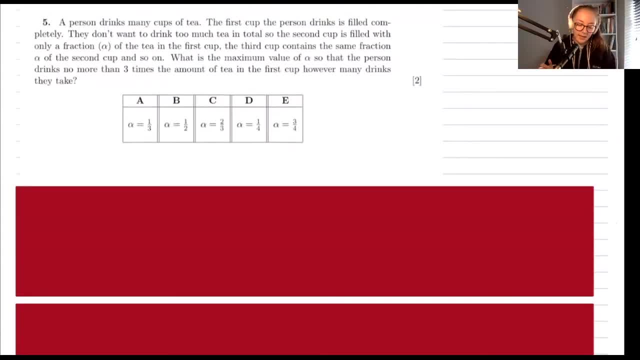 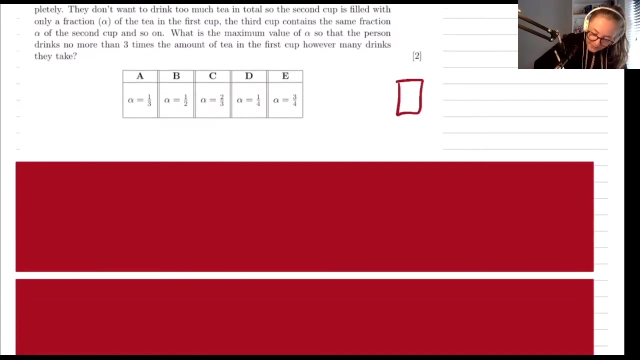 so one downwards plus the infinity of each term. so if a person drinks three cups of tea, this makes the наб that we have wrong, but the term that i studied here now of the second cup and so on. so we start with a big cup, then we say take maybe half, and then 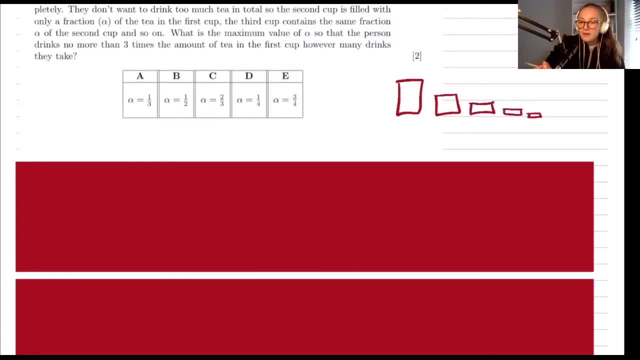 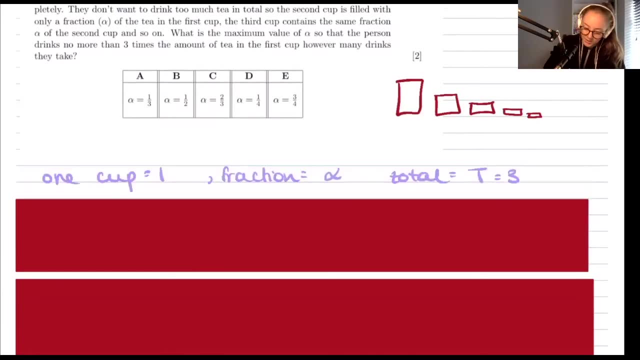 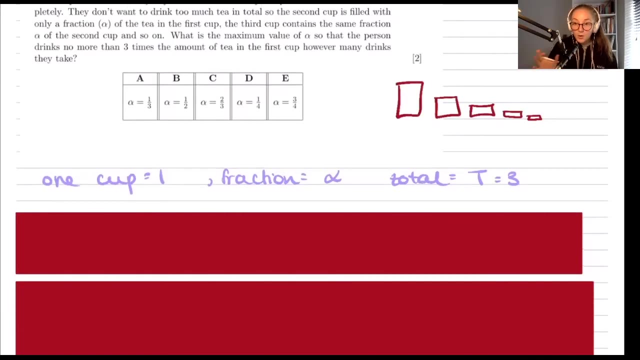 we take half of that and half of that and so on, and it gets smaller and smaller and smaller. so this suggests that we have a geometric series. oh, and the question asks: what is the maximum value of alpha, our common ratio, so that the person drinks no more than three times the amount of? 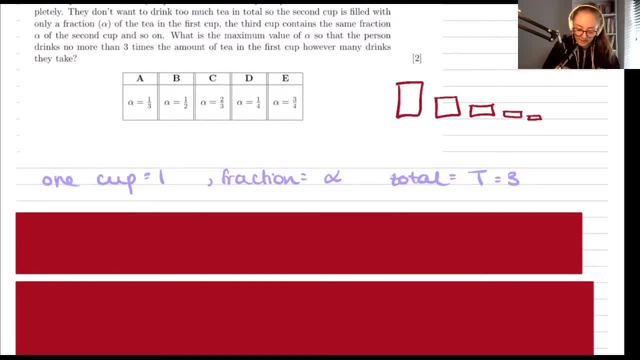 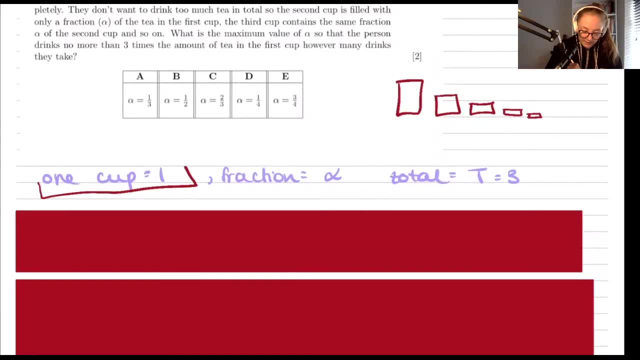 tea in the first cup, however many drinks they take. so, extracting information from here, we'll just say that one cup is one, we'll say that the fraction, or the common ratio is alpha, and then our total- we'll call it t- will have to be three at the end. 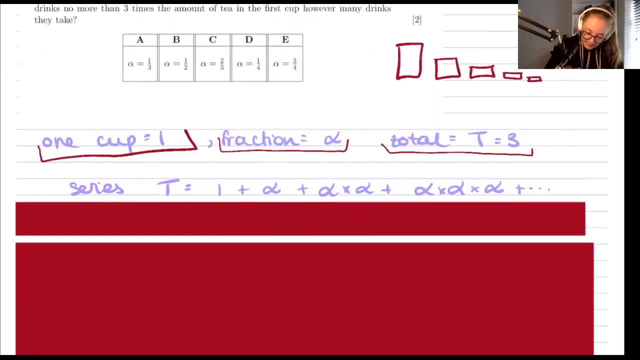 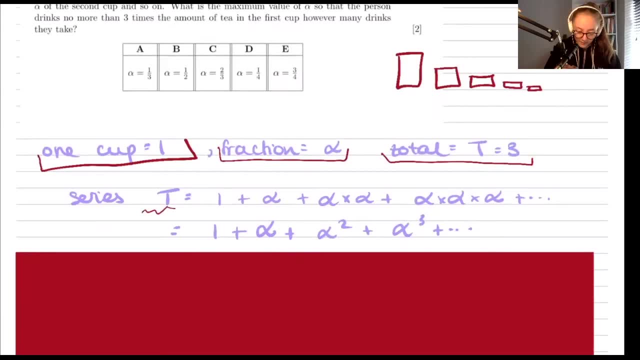 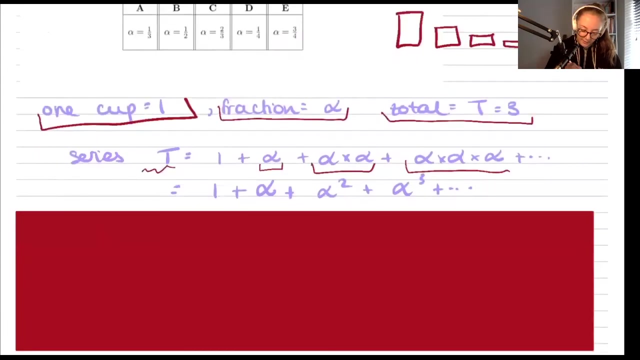 so our series is going to look like this. so our total is one. so our first cup of tea plus one times the fraction. so a smaller cup of tea plus one times the fraction times the fraction times, one times the fraction times the fraction times the fraction, and so on until we end up with this. 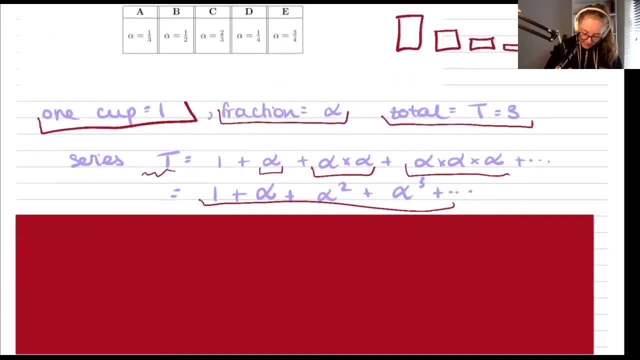 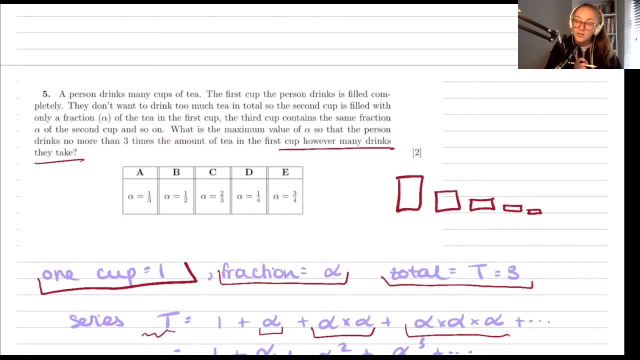 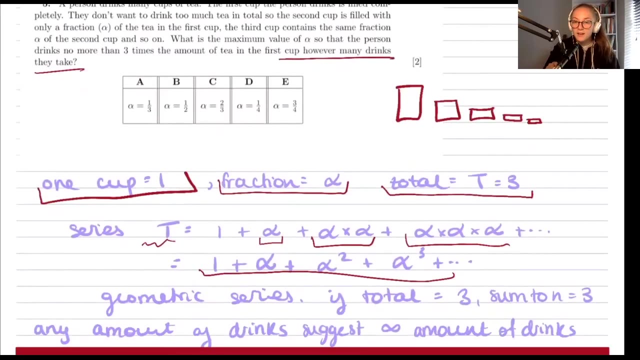 series which looks similar to the one that we had earlier. but there's also another key thing to take out of this question, and it says however many drinks that they took. so however many drinks as they like implies they could have one cup of tea, five cups of tea, ten cups of tea, a hundred cups of tea, a thousand cups of tea. 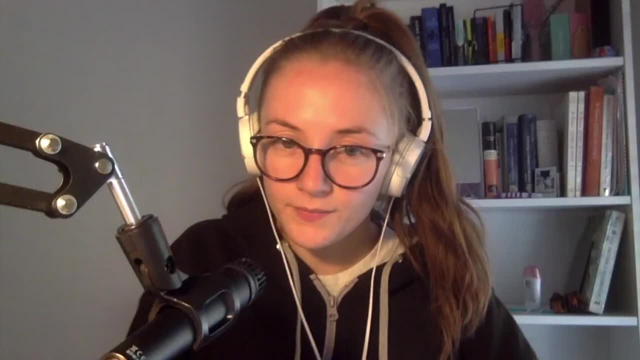 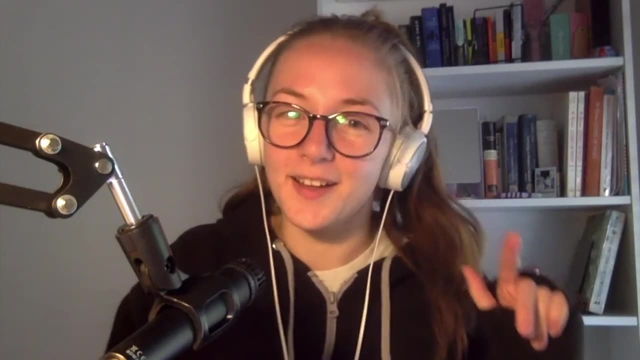 billion cups of tea. infinite amount of cups of tea. hi, this is editing me. congratulations if you made it this far, by the way, but i should have specified that the cups of tea were shrinking after each cup. so we're essentially saying: if we have an infinite amount of cups of tea, 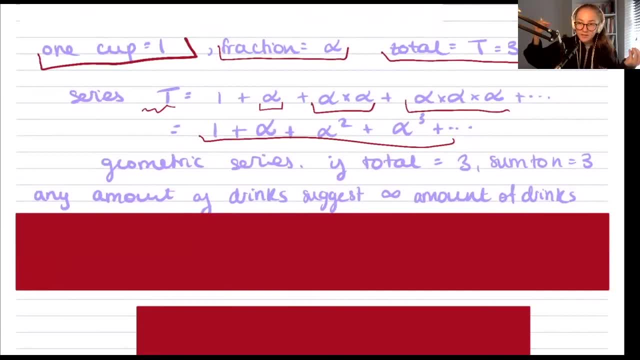 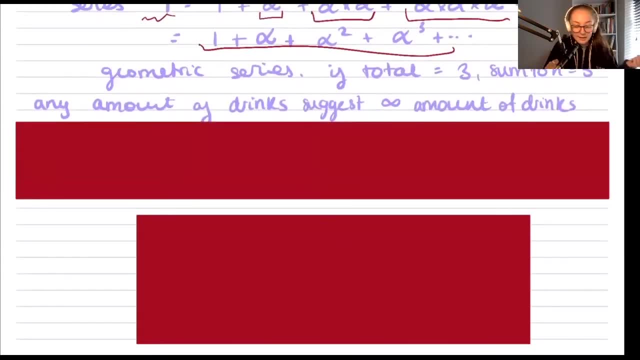 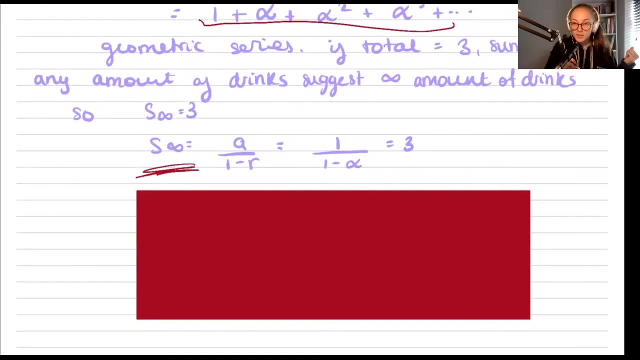 some unspecified massive amount. um, how can we make sure the total is still three or less? so you've probably guessed that we're going to be using the equation that we looked at earlier, and that is sum to infinity, which is a over one minus r. also, just, uh, to mention, you won't? 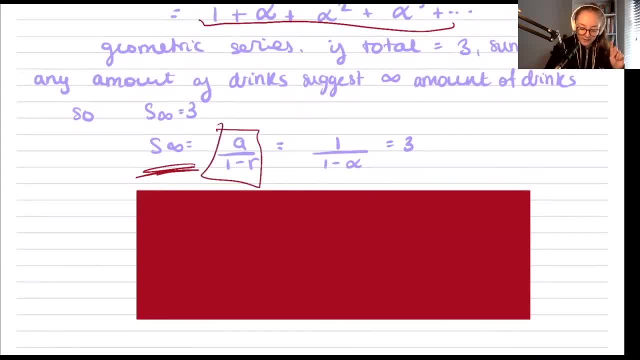 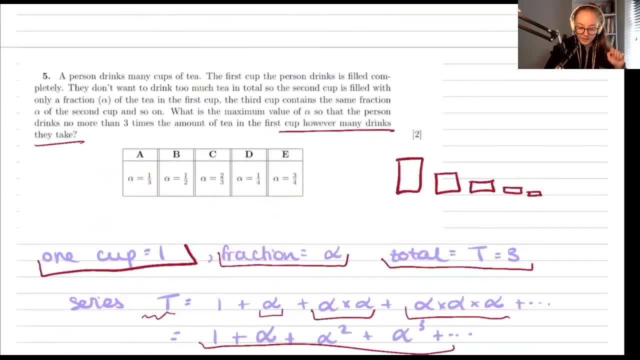 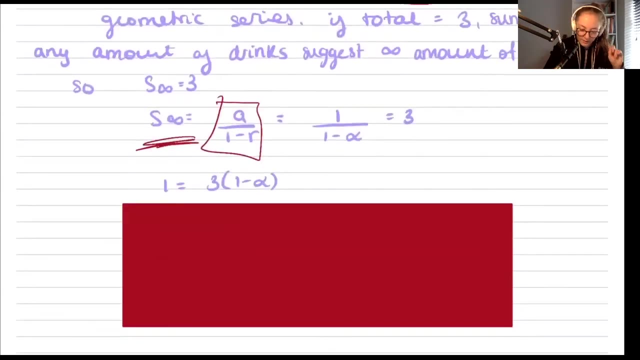 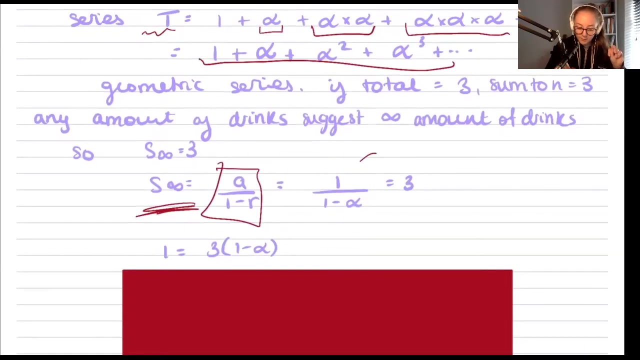 be given these equations. so it is worth memorizing this equation, this equation and this equation if you don't already know them. so we're saying the sum to infinity has to be equal to three or less. so if we stick in our values, um a was one and then our common ratio was alpha, so we start with one. 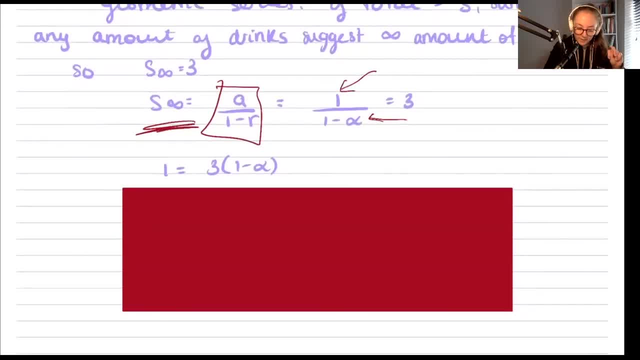 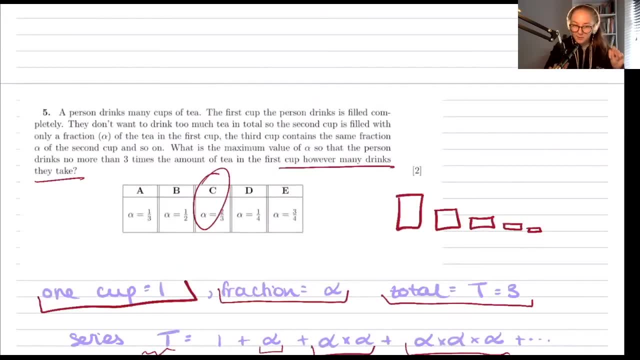 cup of tea. our common ratio here was alpha. then we can rearrange this to get a value of alpha which is two over three, and thankfully that is one of our options. here it was c. okay. next is a kind of typical equation, which is the sum to infinity, which is a over three, and then our common ratio. 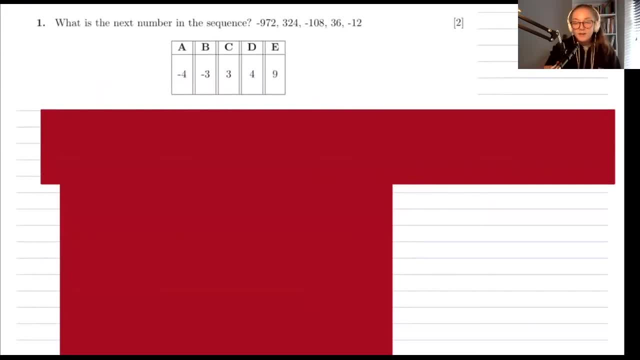 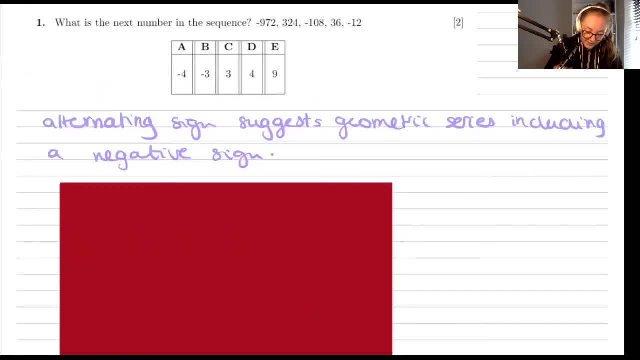 which is a over three, and then our common ratio, which is a over three, and then our common ratio. example of a sequence: question and um. these can sometimes be in the form of an arithmetic or a geometric series, so definitely keep that in mind. um, this one here. as we see, here we have an 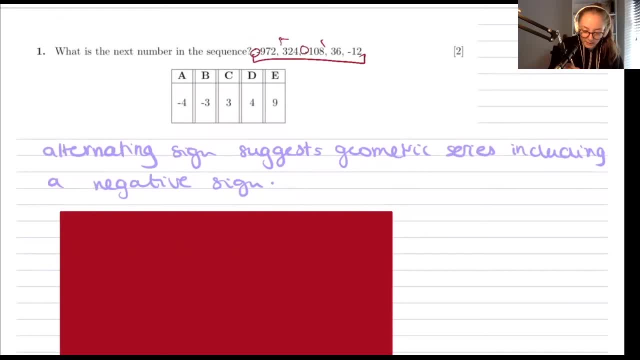 alternating sign. so we have a minus, we have a plus, we have a minus, a plus, a minus. so, just as a pointer, that normally suggests that you have some kind of a geometric series where you're multiplying by a minus number, because for this one we've times by minus something. 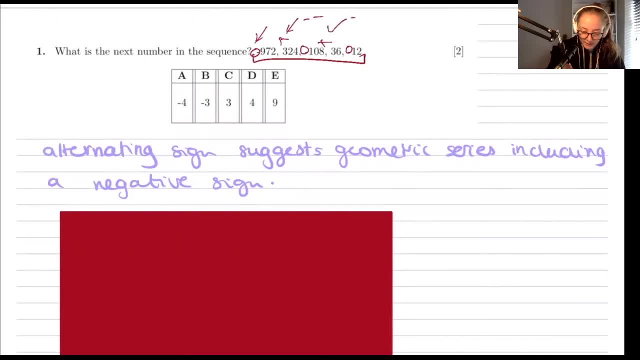 and then this one is a minus, minus, and this one is a minus, minus, minus, and then this one is a minus, minus, minus, minus. So minus, minus is a plus, minus, minus, minus is a plus times a minus, which is minus, and then a minus, minus, minus, minus is a plus times a plus, which is still a plus. 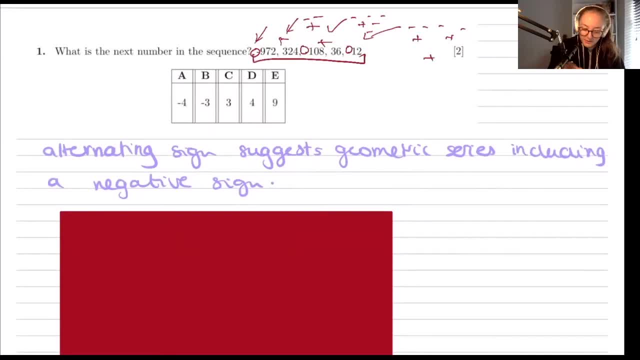 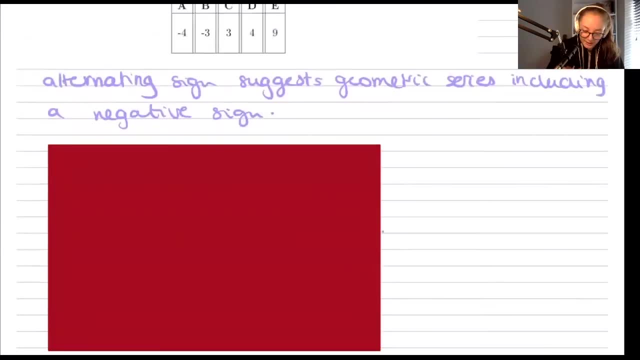 And that lands us with alternating signs. If that was really confusing, I'm sorry. So yeah, this is suggesting that we have some kind of a negative sign in our geometric series. So if it's a geometric series, what might we be multiplying with each time to get the next one? 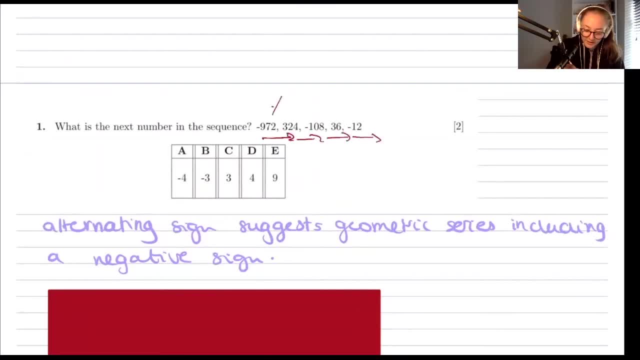 Well, if you have your calculator at hand, it's worth just dividing one value by another to see what you get. So 972, or minus 972, divided by 324, what we get is minus 3.. So what if we try that again? So 324 divided by minus 108, what do we get? 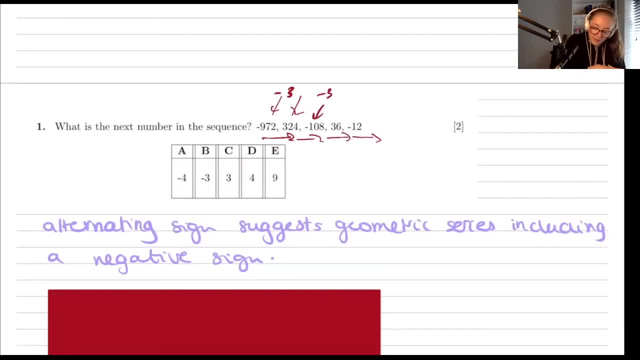 Minus 3.. And minus 108 divided by 36, what do we get? We get minus 3.. 36 divided by minus 12, what do we get? Minus 3.. So this is suggesting that we are dividing by minus 3 each time. 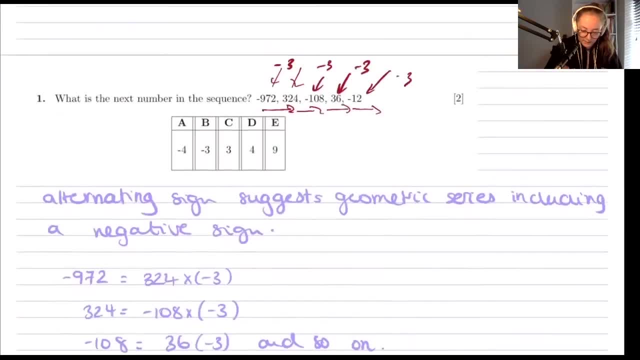 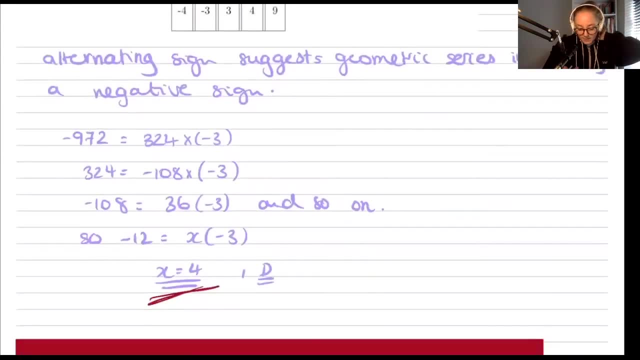 So our next number in the sequence will be minus 12 divided by minus 3, which is 4.. And luckily, that is one of our answers- It is D, So I would say, if you're struggling to see that, that's OK. 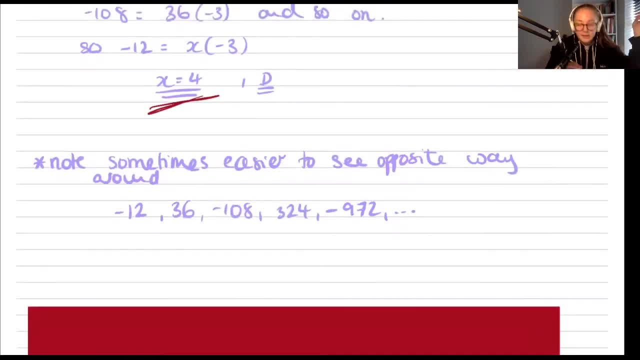 But you might find it difficult to see that. So I would say, if you're struggling to see that, that's OK, But you might find it difficult to see that, So try and write it backwards and see if it's easier to see the progression. 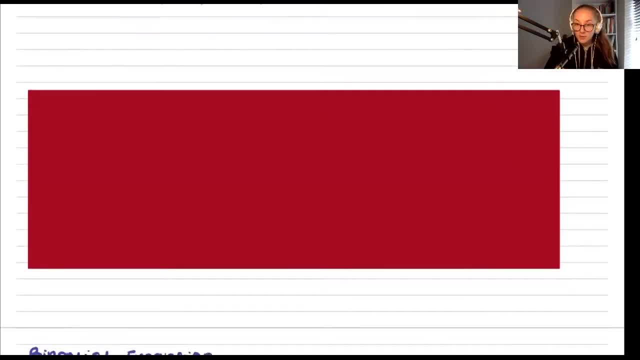 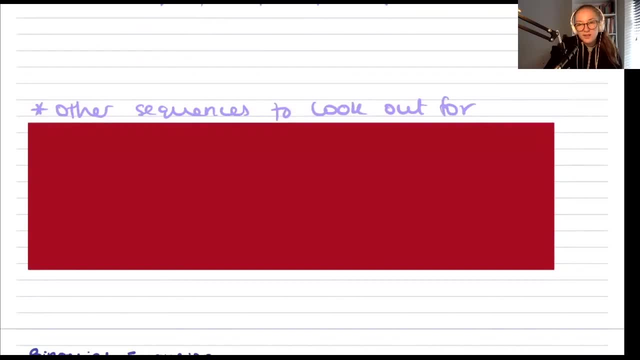 So, when it comes to sequences, there are a few other sequences you should probably be aware of that could come up, because these ones will not look like a geometric or an arithmetic series. But keep your eye out for a sequence of primes. These might not always start at 1.. 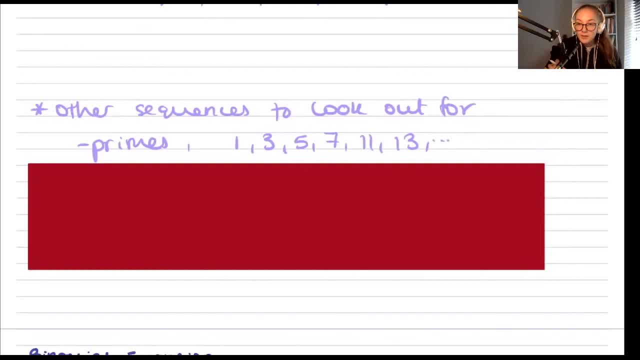 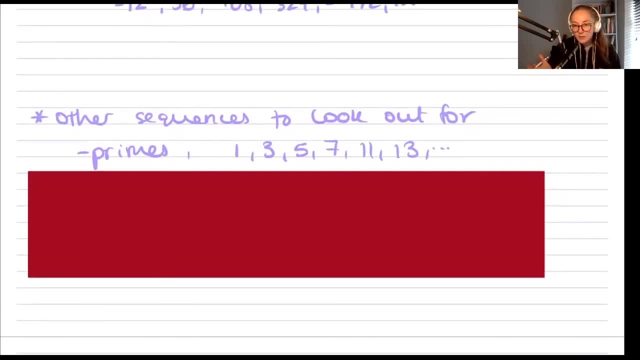 But you should know, a prime number is one which can only be divided by itself and one which can only be divided by itself. So 1,, 3,, 5,, 7,, 11,, 13.. These are all prime numbers. 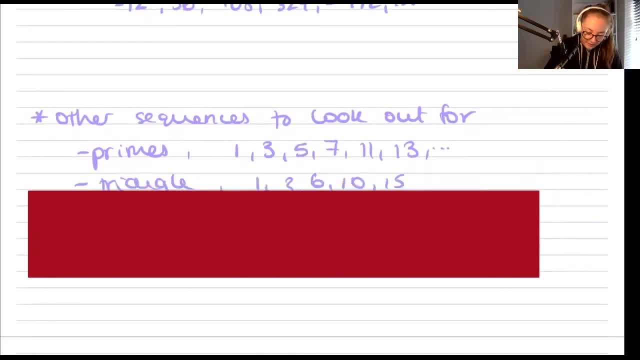 So it might be a sequence of prime numbers, Triangle numbers. So these are ones where you have 1,, you have 2, plus 1.. You have 3 plus 2 plus 1.. You have 4 plus 3 plus 2 plus 1, and so on. 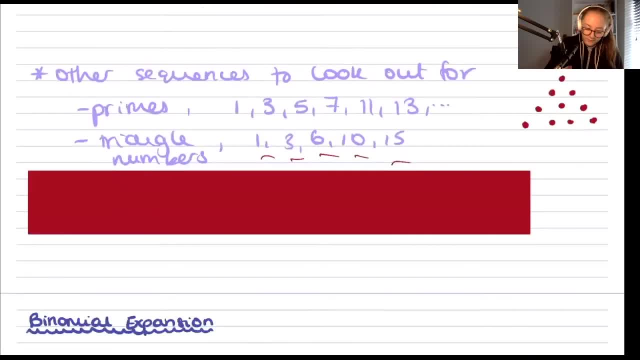 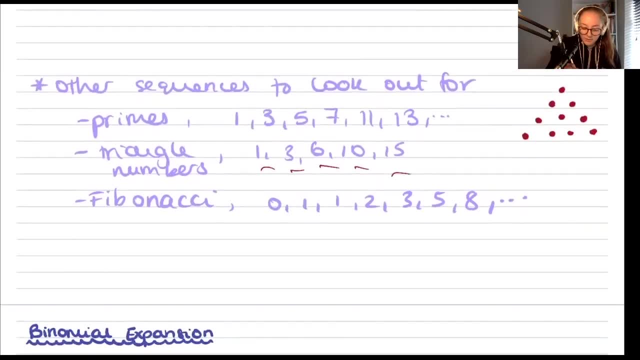 So 1,, 3,, 6,, 10,, 15, and so on. Or another one to look out for is a Fibonacci sequence, And a Fibonacci sequence sequence is one where you add the previous number to your current number to get the next number. 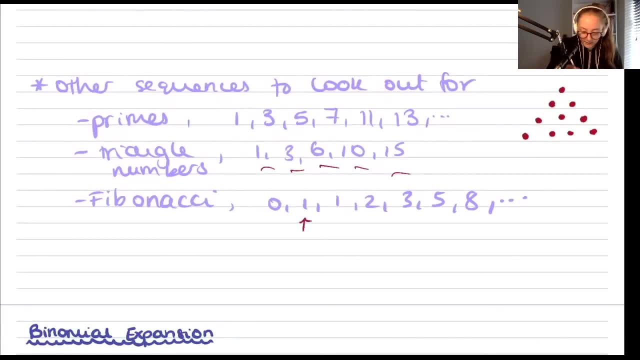 So if we look at one here, if we add naught to one, then we get one. So the second term, if we add one to one, we get two. And then this term here, if we add one to two, we get three. 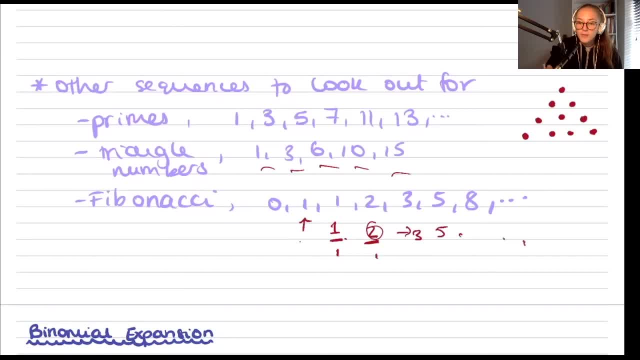 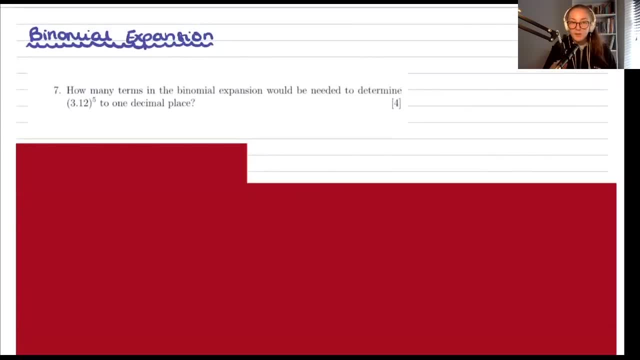 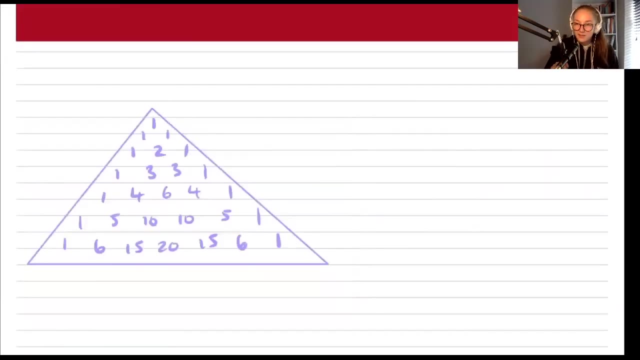 And then, if we add two to three, we get five, and so on. So these are just different sequences that you should keep your eye out for. Okay, so my final topic in this video is binomial expansion, And I'm sure you've all done binomial expansions in school. You're probably all familiar with this. 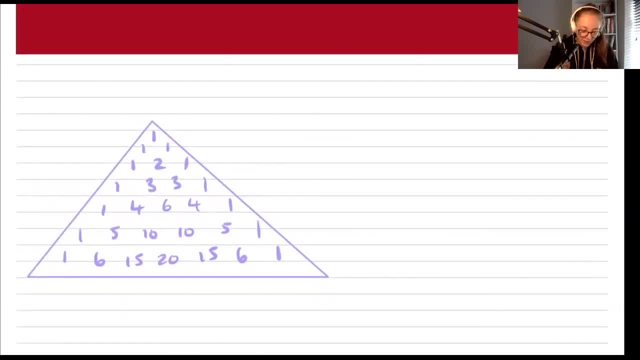 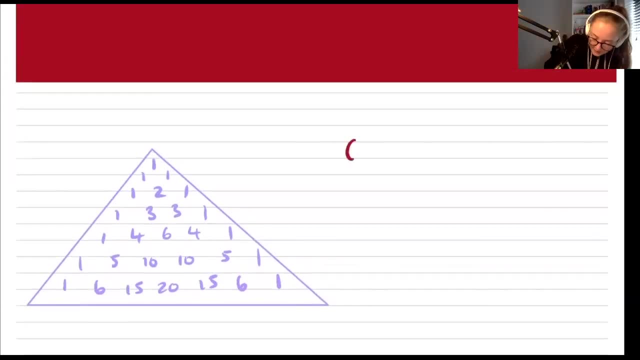 triangle. But these are your binomial coefficients. This is how I've always remembered how they are. But if you can't remember what this means, then say: we have x plus y to the power of two. You probably know that if we multiply out this bracket, we get x squared plus 2xy plus y. 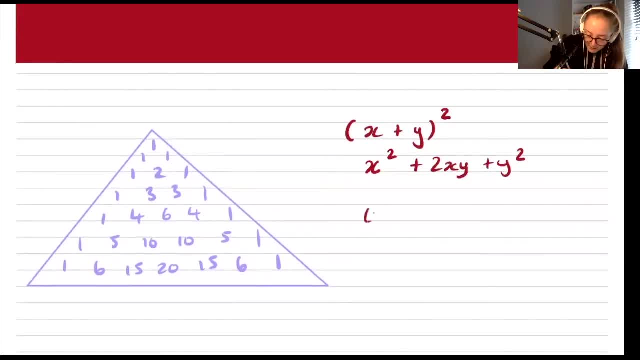 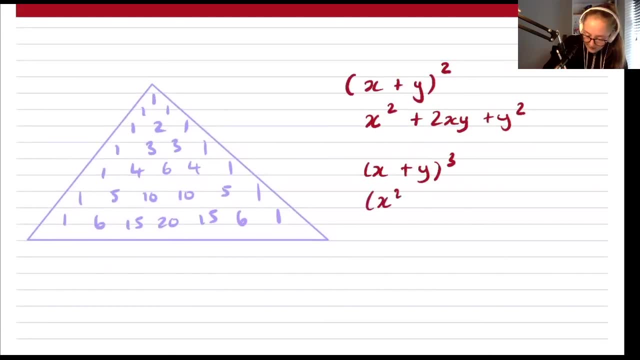 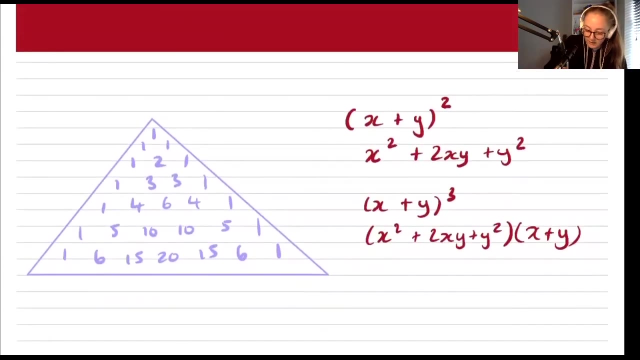 squared Simple. So if we have x plus y to the power of three, this will take a little bit more work, but you can do the same thing again and multiply that by x plus y, and then multiply all these terms and then you'll get x. 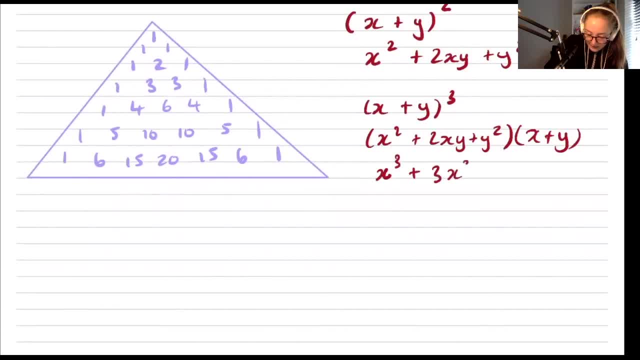 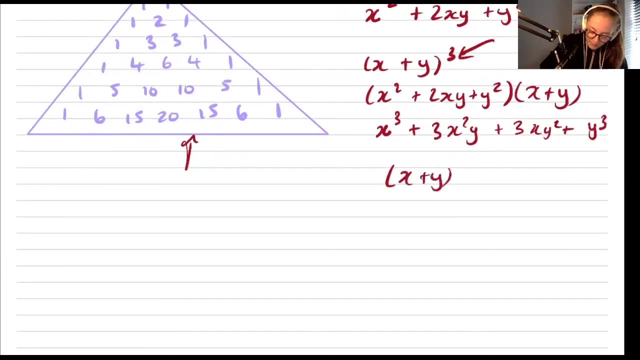 cubed plus three x squared, y plus three, x, y squared plus y cubed. But obviously the higher and higher this power gets, the more complicated this will be. So this is why we use the binomial coefficients, because we can say: okay, so we have x plus y. to the power of six we can look. 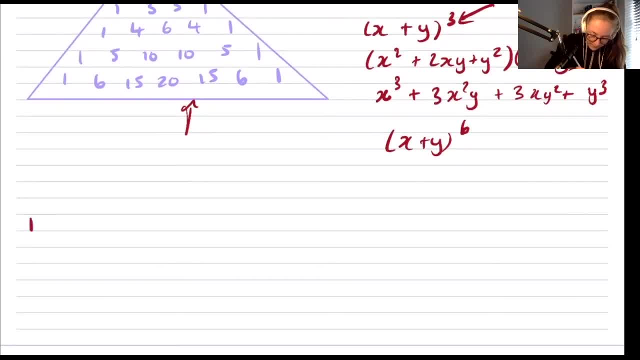 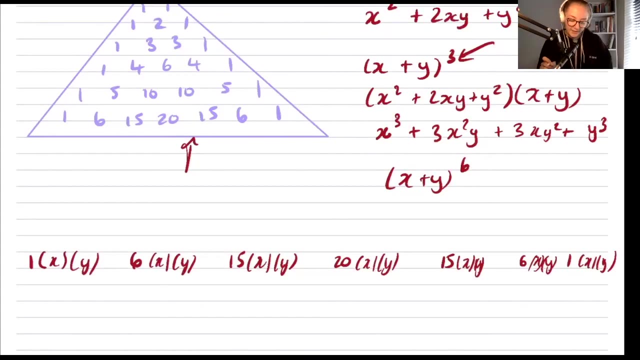 at the binomial coefficients to say: well, we'll have one, Six, 15,, 20,, 15, six, one is our coefficients. And then, if we look at the pattern of what's going on here, we have x, y, x, y. Okay, so here we have our different terms, and then we just decrease. 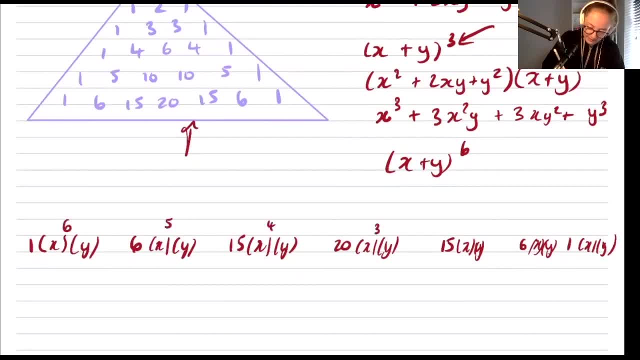 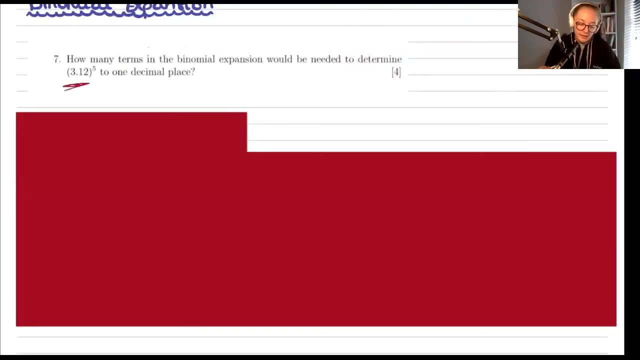 the power each time starting at the power of our bracket. But I'm sure you already knew how to do binomial expansion. So this question now is asking us how many terms in a binomial expansion do we need to get 3.12 to the power of five, to one decimal place.